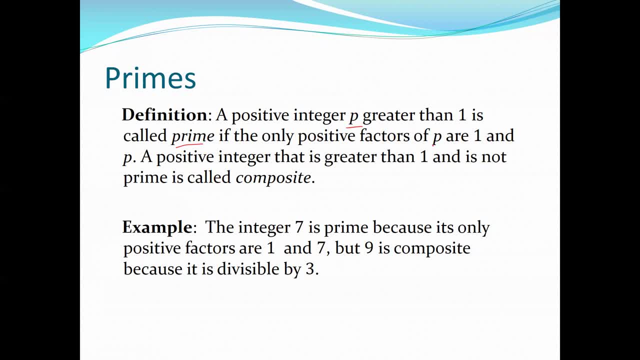 is called a prime if, and only if, positive factors of p are 1 and p itself. right, That mean is, if that positive number, any positive integer, if it can be divisible by only 1 and itself the prime factors are only p and 1, then we call it a prime number, A positive integer. that 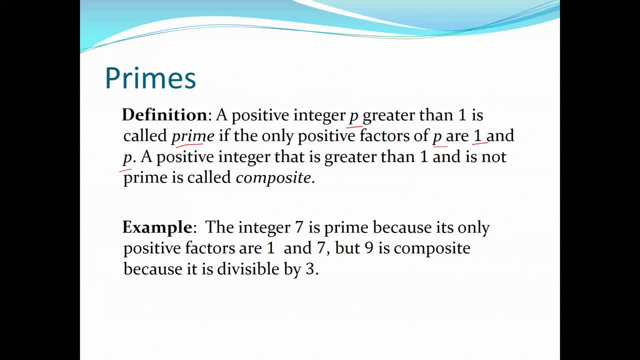 is greater than 1 is not prime, is called a composite. If the number is not prime, then it is called a composite number. So like, for example, the integer 7 is prime because it only has positive factors 1 and p. So if the integer 7 is greater than 1, then it is called a composite number. 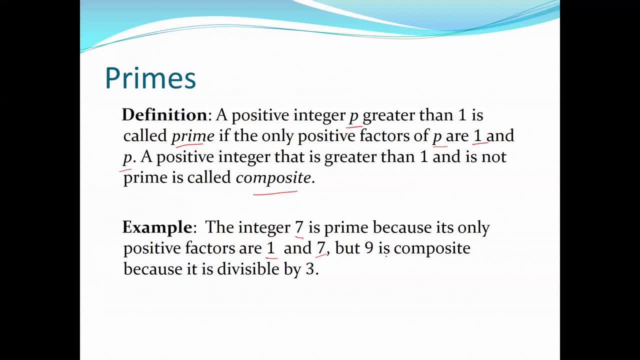 So all the numbers that are not prime are called composite numbers. Then the element can be bullshit and it is divisible by 1 and 7, right, So? but 9 is not composite. 9 is the composite is not a prime because it is divisible by 3.. So 9 has the factors 3 into 3, right. 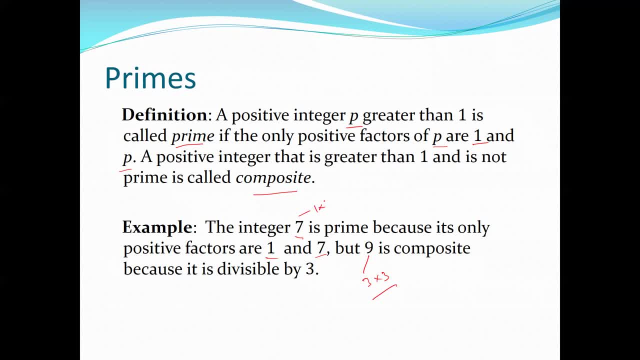 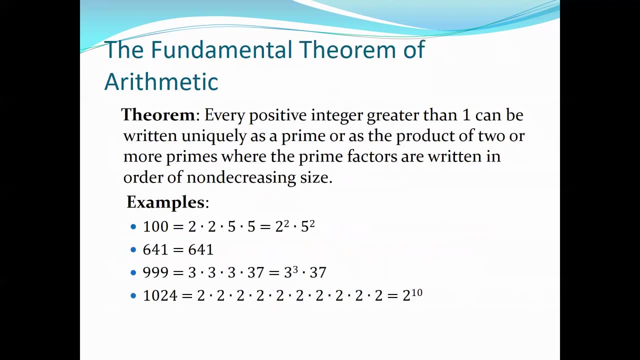 So, but 7 has the factor only 1 into 7.. So all the numbers that have the positive factors of itself and 1 are said to be the prime number, and all those numbers that are not prime are called composite numbers. So the fundamental thing to understand here is that the prime numbers 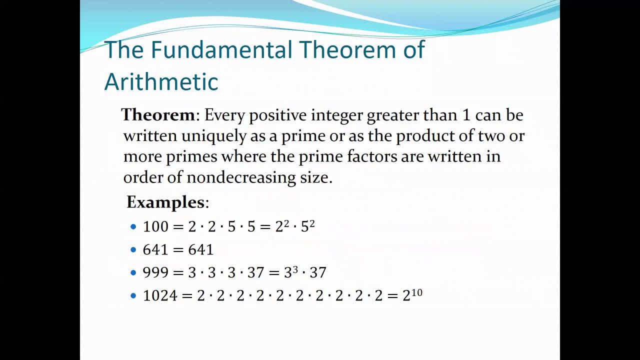 and the less d part of the number are essentially equal to zero and zero. okay, So the property of theorem of the arithmetic, every positive integer greater than one can be written uniquely as a prime or as the product of two or more primes. so remember any, i mean any integer greater than one. 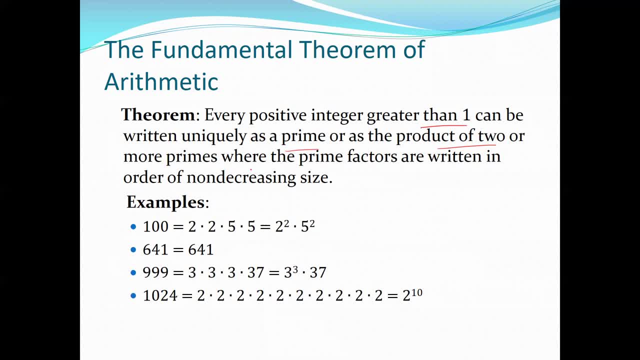 can be written as the prime or product of two primes, where the prime factors are written in order of non-decreasing order. for example, 100- 100 could be written, and i mean we can find the factors of the hundred, prime factors of the hundred. so we know that, how we can do that. two: 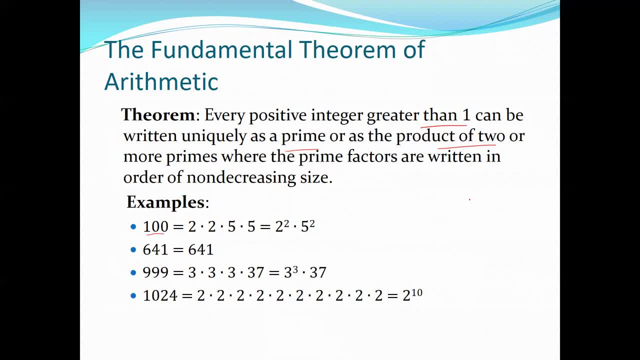 into two, into how we can do that, if you remember from your early schools. if you are interested to find the prime factors of hundred, just divide it with two right the the smallest number right greater than one, then it will become 50. then divide it by two, you will get 25 right and keep. 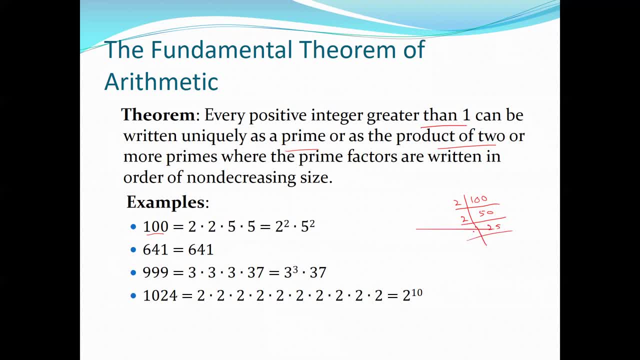 on doing this, then you cannot divide this 25 by 2, you need only 5, and 5 times 5 is 25. then you can write it in terms: 2 into 2 into 5 into 5, right, or 2 power 2 into 5 power 5. 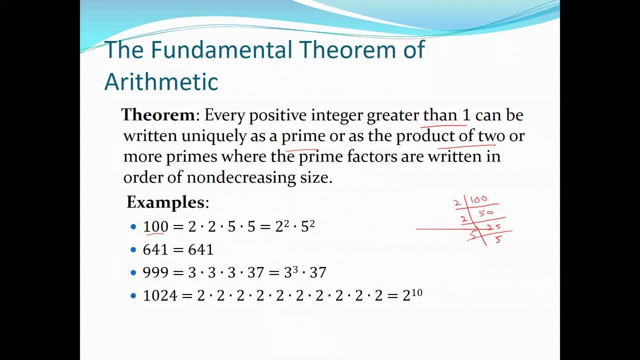 similarly, 641 does not have any prime factor, uh greater than i mean. this is uh the not factor, except uh 6, 641. so 999, 999, you can write it 3 into 3, into 3, into 37, right? so you can always. 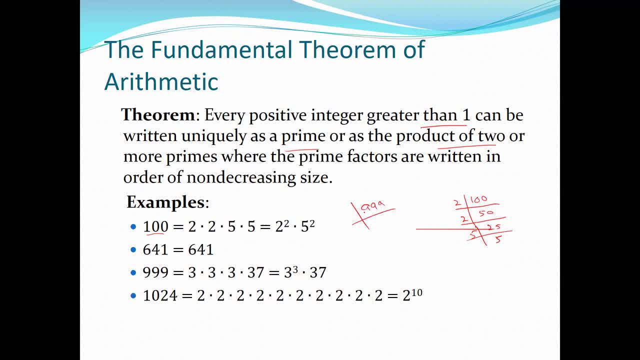 see that 999 you can divide it with. you cannot divide it by 2. then 3, 3, 3 and then you can divide it with, i mean again with 3, that 1, 1 and 1. again you can divide it with 3. 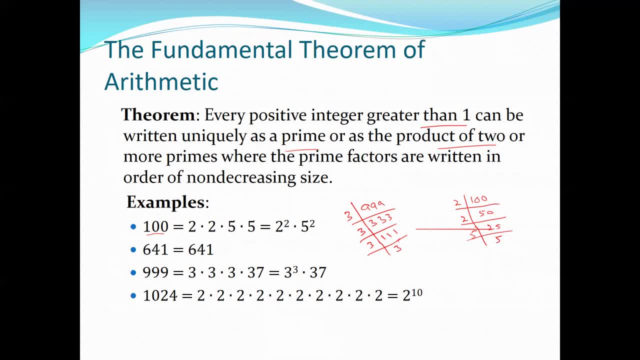 and then this will become 3, 3s are 9, and then 3, 7s are 21, so 3, 3, 3 into 37, 37. you cannot divide it further, so that's how you can- i mean, uh, we can represent any, uh, the positive integer greater. 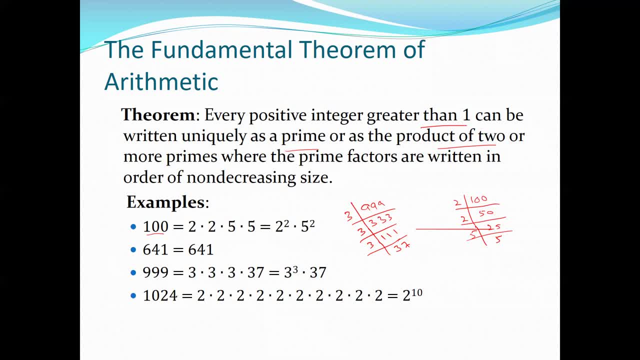 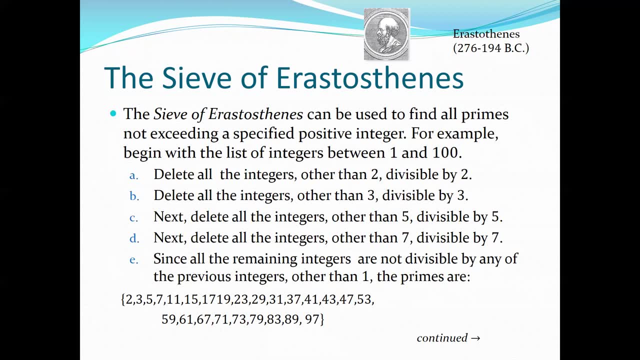 than 1. we can write it with the product of 2 or more prime prime numbers, the sieve of- uh, rough essence, this is a formula, this is an algorithm in order to compute the first n prime numbers right, so the sieve of retrosense can be used to find all prime. 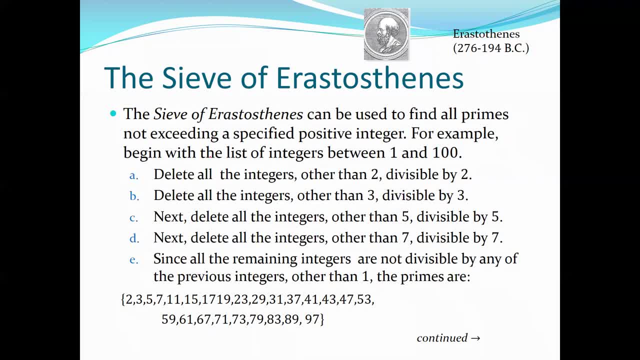 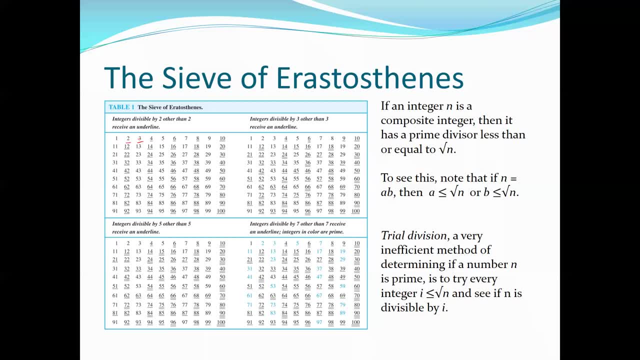 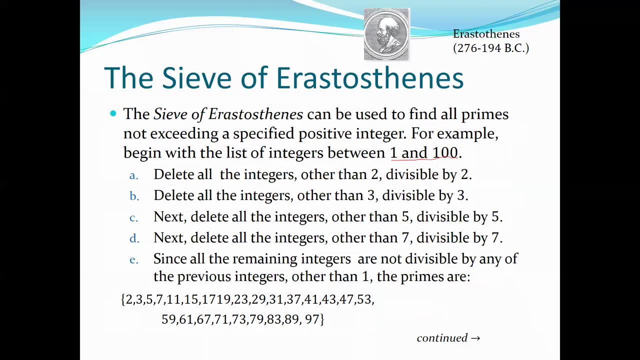 find the multiples of 13, and you will do that. so this is the algorithm, and when the algorithm will end up, you will see only the prime numbers are remaining between the list. so now let's see here. so what you are going to do: delete all the integers other than 2 divisible by 2, i mean. 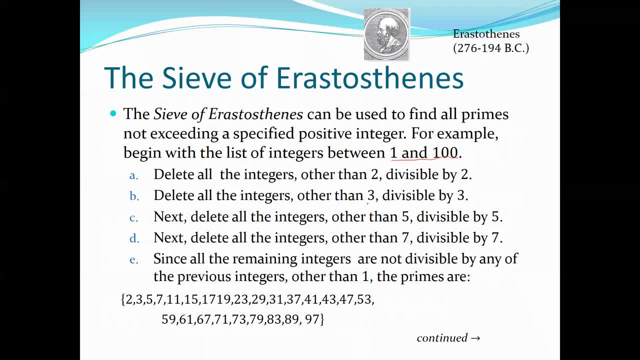 multiples of 2. right, so delete all the integers in the third next phase other than 3 divisible by 3. all the integer divisible by 5. all integers divisible by 7. why? because these are the multiples of these numbers. so, since all the remaining integers are not divisible by any of 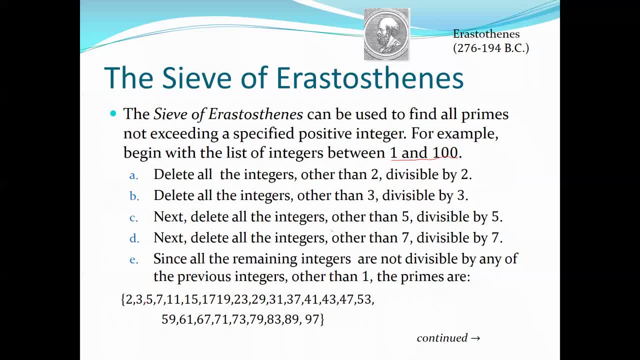 the previous integer other than 1, so these are the prime. for example, 2, 3, 5, 7, 11, 15, right um 7, not 15. actually 15 is not in the list, right, this is the mistake here. 15 is not in the list. 17, 19, 23, 29, 31. 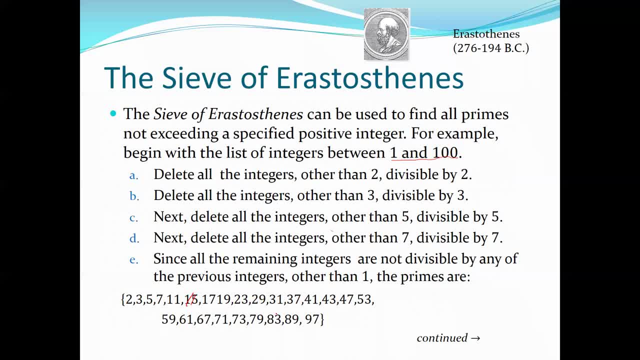 37. so these all are the prime numbers from 1 to 100. so you gave a list of numbers to save over a sense that is 1 to 100 and then it it will delete all the composite numbers from the list. by the multiple factors i mean multiples of 2, then multiple of 3, then multiple of 5, then multiple. 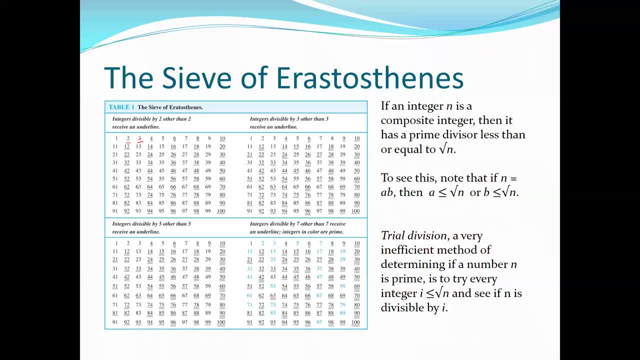 of 7 and so on. right clear. so then it turns out that, uh, this is the. i mean there is a complete, this is the complete algorithm. you can. the algorithm is given in the book, so you can. uh, you can see that if an integer n is a complete algorithm, you can see that if an integer n is a, 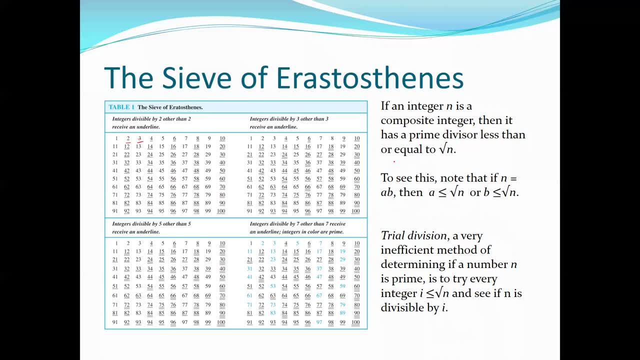 composite integer, then it has a prime divisor less than or equal to the square root of n. for example, if n is 16- right, so 16 is. n is a composite integer, then the prime divisor of 16 would be less than the square root of n. so you can see the: the divisor is less than a prime, that is. 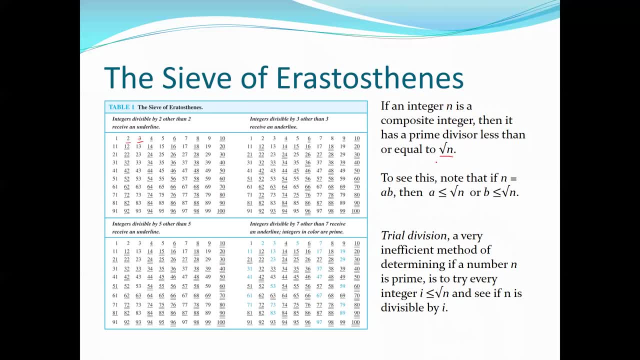 i mean if you take the square root of 16, that is 4, and then the prime, the divisor of this would be less than uh 4. that is obviously see the 2 is, the divisor of 16 is 2.. That 16 will be deleted in first phase, first pass. 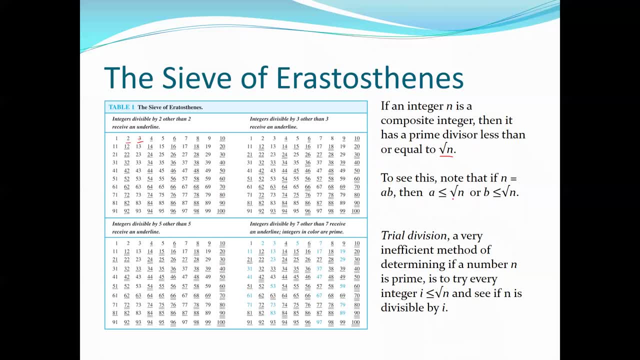 To see this. note that if n is equal to a, b, then a would definitely be less than or equal to square root of n and b is definitely less than or equal to square root of n. So that means in the trial division: 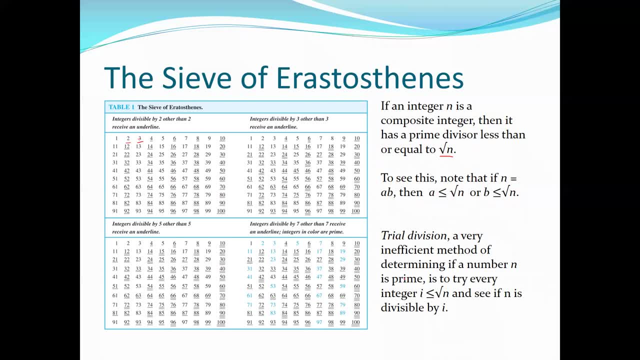 a very inefficient method of determining if a number, n, is prime is to try every integer i less than or equal to n and see if n is divisible by i. So, instead of dividing the list by all numbers, we actually see whether, for example, if we talk about 100,. 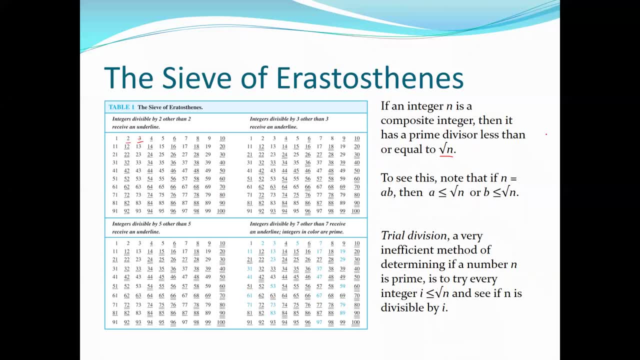 100 would be the square root of 100. We need to find out the square root of 100.. So if you compute the square root of the 100, that would be 10, right. So that means that the square root of the 100 would be 10.. 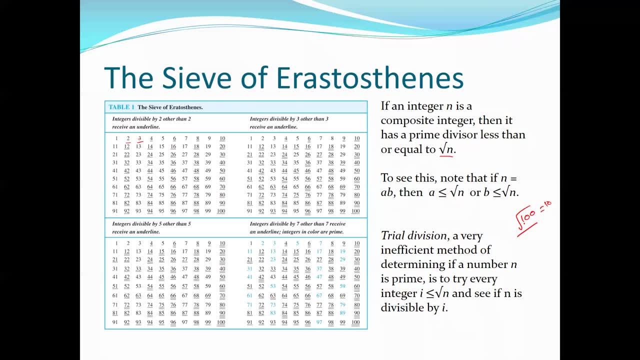 That means the divisor devising factor of 100 would be less than 10.. For number prime value that is less than 10.. Then it turns out that you already have gone through the list from until 7, from this list, right? 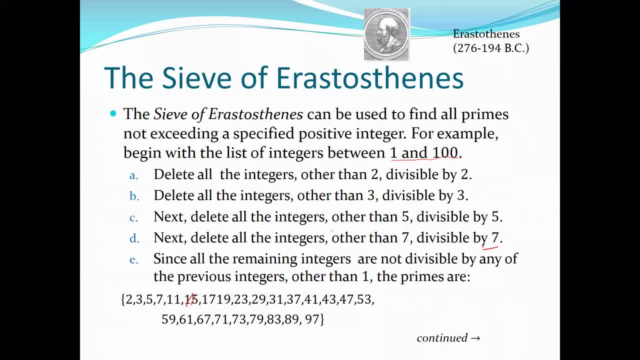 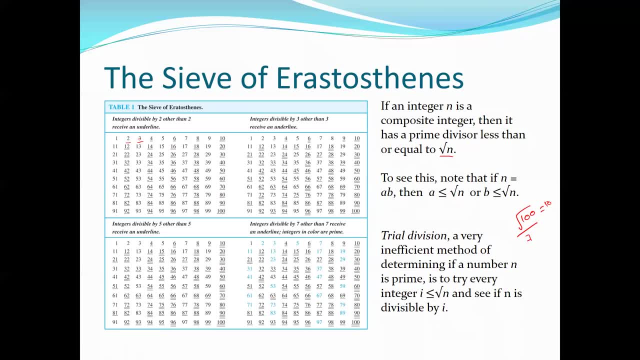 Divided by 7.. But the next prime would be 13 or 11. So then 11 is greater than 10.. So you do not need to check the multiples of 11 at all. So you need to. that means you will see. 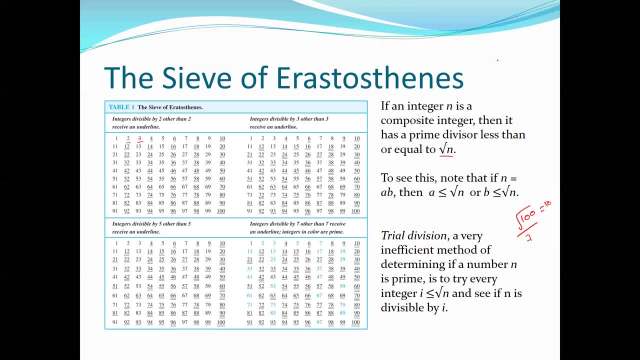 the last number in the list, that is, whatever is in the list, to take the square root of that And before that, the value of that square root, we will be dividing the list. the number less than that, the square root of the 100, right. 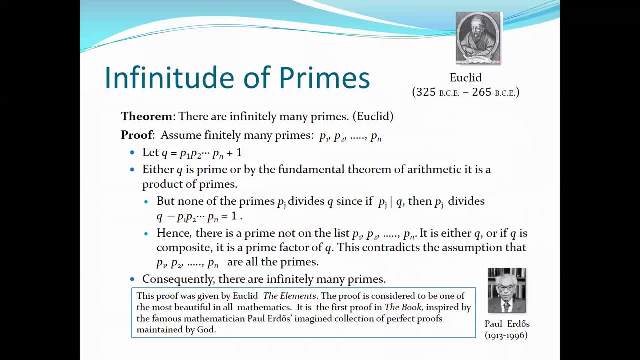 Okay Then, infinitude of the primes. So the theorem is: there are infinitely many primes. This theorem was given by the Euclid In in in 325 BC, right? So how you can prove that there are infinite number of primes. 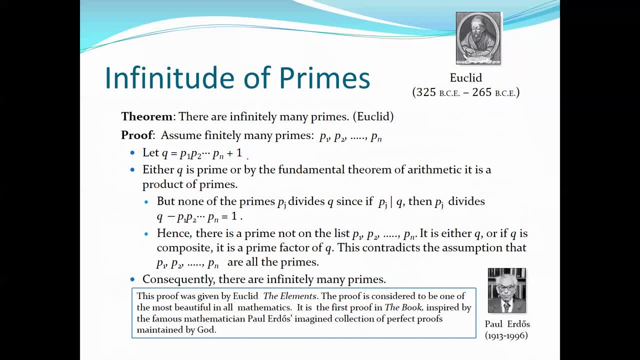 So let: Q is equal to P1,, P2, up to Pn plus one. So these are the prime numbers. Either Q is prime or, by the fundamental theorem of the arithmetic, it is a product of primes. We know that either Q is prime or it is the product of prime numbers. 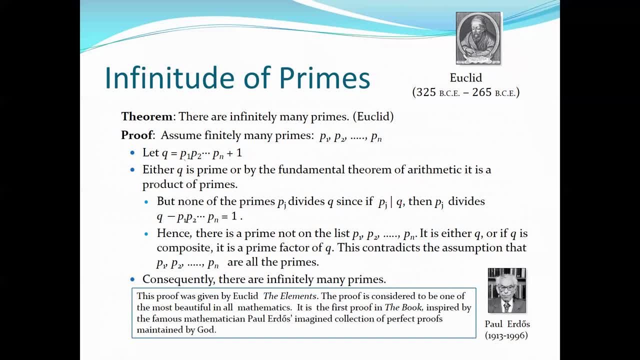 but none of the prime. PJ divides Q. since PJ divides Q, then PJ divides Q, So we know that Q minus all these primes equal to one, since this is plus one. So hence there is a prime not on the list. P1, P2 up to Pn. 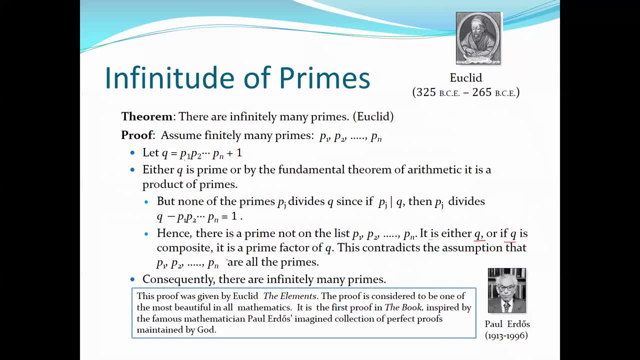 It is either Q or if Q is composite, it is a prime factor of Q right. So this contradicts the assumption that P1, P2 all are the prime number. So that means one of them is not the prime right. 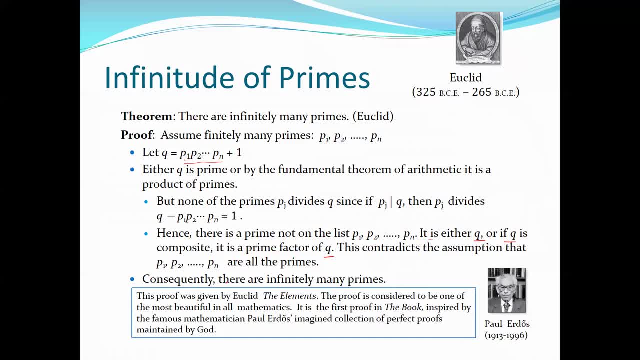 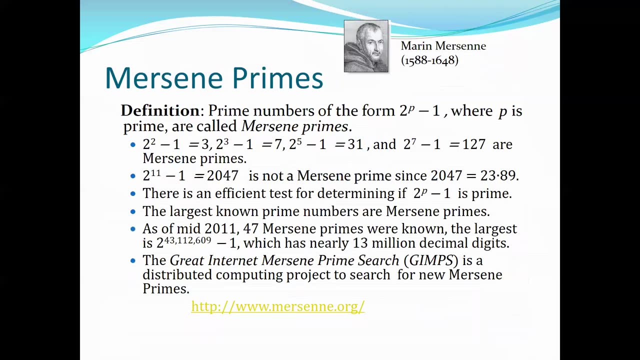 So consequently, consequently, there are infinitely many primes. So it is proven that there are infinitely many number of primes. So this proof was given by the Euclid. So I mean so to remember this, we have the infinite number of primes, as we have discussed in the previous videos as well, in the Herbert's Hotel example. 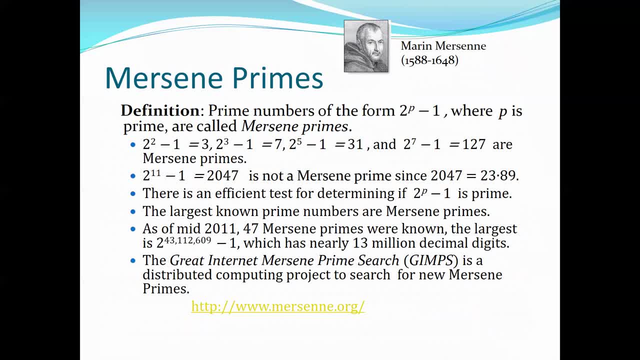 where we see the infinite number of rooms with the infinite number of passengers, infinite prime numbers, right? Then another concept is the Mersant's prime. So Mersant was basically a mathematician. So prime numbers of the form two power P minus one. 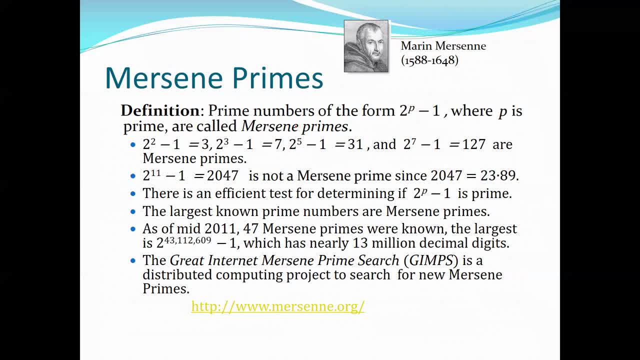 where P is prime, are called Mersant's prime. So what happens? basically, if you take two square minus one, that is three, two cube minus one, that is seven, I mean you just take the power of, I mean two, to the power of any prime number minus one would return into prime. 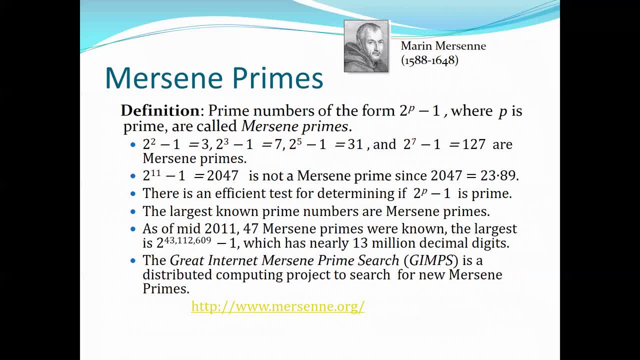 For example, you are going to take the two. two power seven. seven is a prime number. two power seven, That is 128 minus one, That is 127.. That is again a prime number, right? So two power 11,. 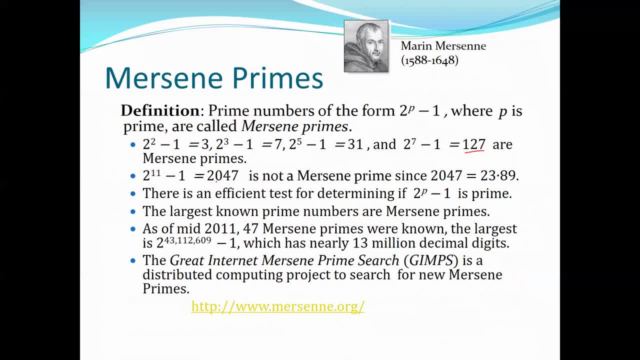 for example, that is 248 minus one, That is 247.. That is again a prime number. So prime number is. so the prime prime numbers are the Mersant primes are. it says two to the power of any prime number minus you subtract one from it. 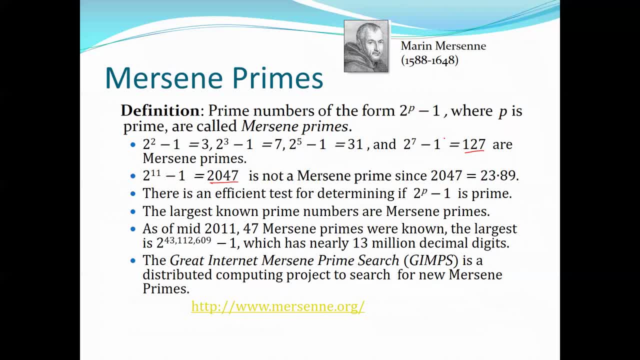 Take the power of two- two to any prime number and subtract one from it And as a result, you will also get a prime number right. So this was experimented by the Mersant's, and these are called Mersant's prime number. 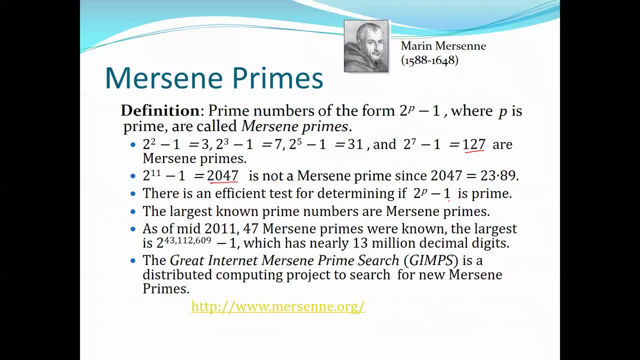 So there is an efficient test for determining two to the power of P minus one is a prime. So we we have already seen that the largest known prime numbers are Mersant's prime number. As of mid 2011,, 47 Mersant's prime number were known. 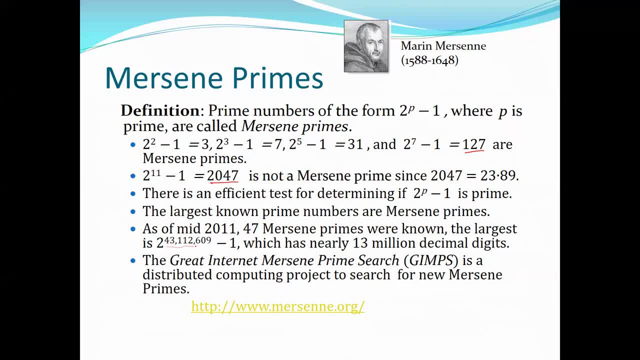 The largest is two to the power of this value right Minus one which has nearly 13 million decimal digits. So the great internet Mersant's prime search- you can go to this website right- Is a distributed computing project to search for new Mersant's primes. 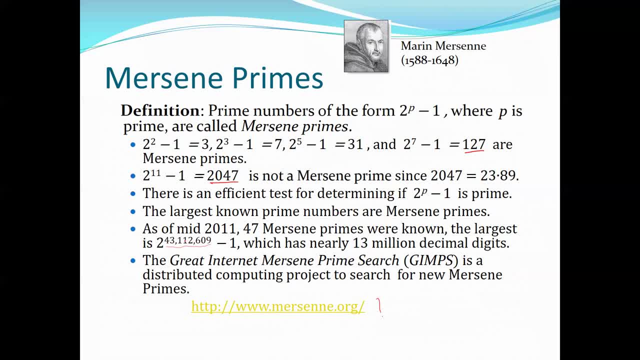 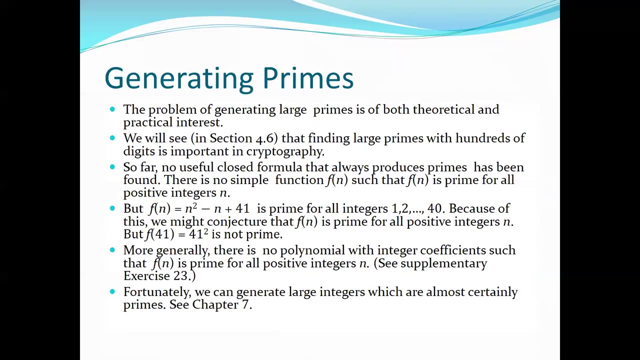 So the Mersant's prime is to take the power of that number. I mean that is the computational limitation. So I mean, how can you compute two to the power of this one? Do we have that machine? So this is the project that actually is looking for the largest primes. clear. 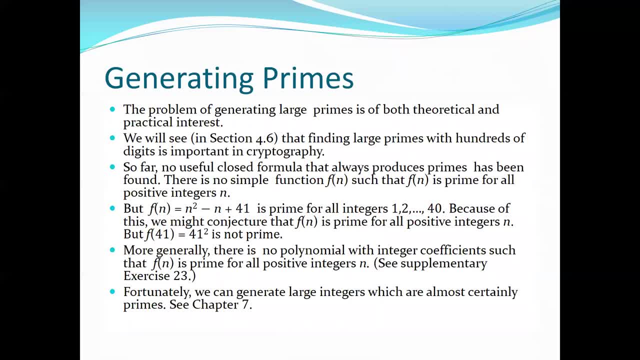 So how we can generate the prime numbers. The problem of generating large primes is of both theoretical and practical interest. We will see that finding large primes with the hundreds of digits is important in cryptography. Obviously, this is important in cryptography, but I will not. 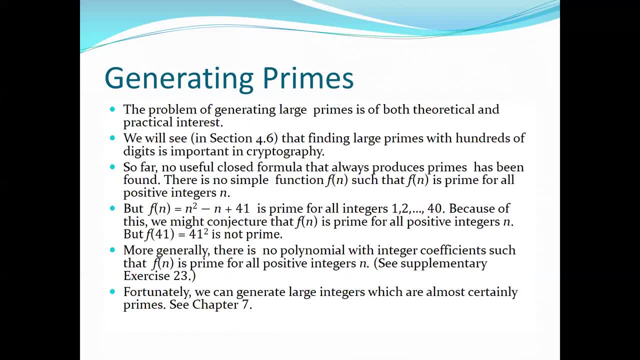 I may not cover cryptography in this in this course, because it it requires a lot of time in order to explain those things, but we'll see. so far known, a useful use formula that always produces prime has been found. There is no simple function FN such that FN is prime for all positive integers. 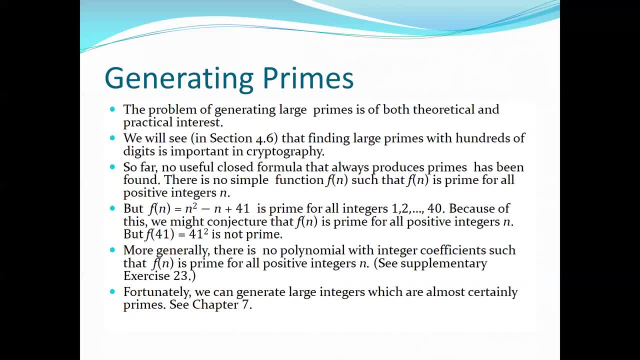 And so we do not have any function like that. So it's not simple or we do not have a useful formula to generate the prime numbers. but then it turns out that FN is equal to N square minus one plus 41 is prime, I mean. 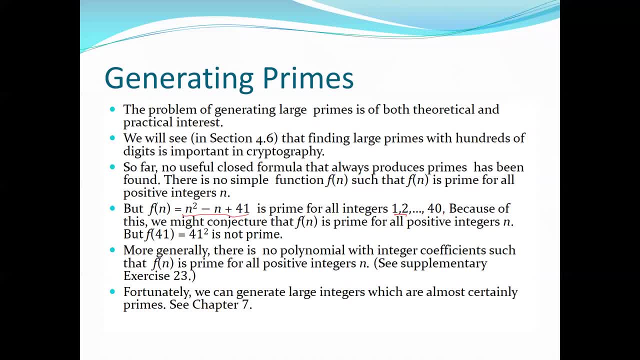 this function is prime for all integers from one to 40, right? So if you substitute the value of one from one to 40, you will get the prime numbers. because of this, we might conjecture that FN is prime for all positive integers. then 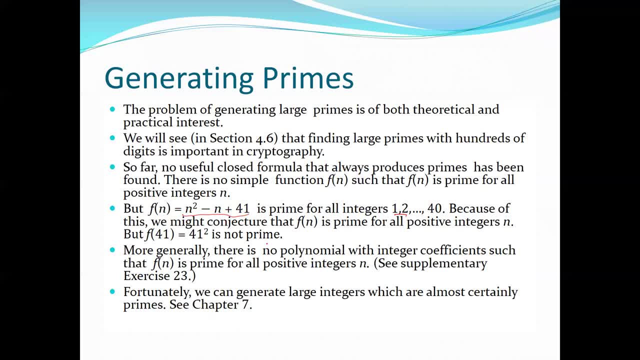 but then F of 41 is not for 41. It is not true. It is true for until 41, but for until 40, I mean up to 48, is fine, but after that it is not true. So more generally, 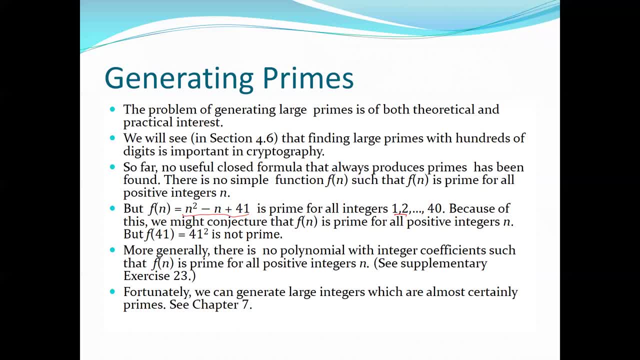 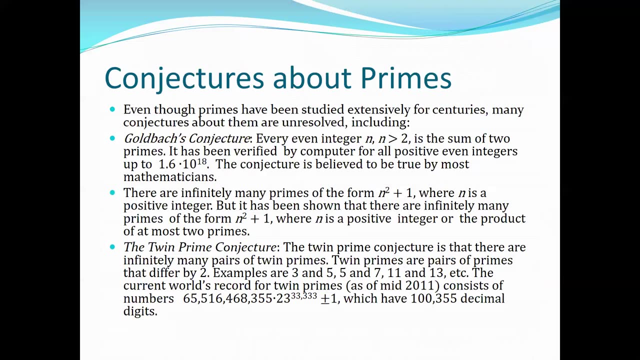 there is no polynomial, a polynomial with integer coefficients such that F of N is prime for all positive integer N. So we do not have any function FN that can return, in that we have a general formula to compute the prime number right. So some conjectures about the prime. 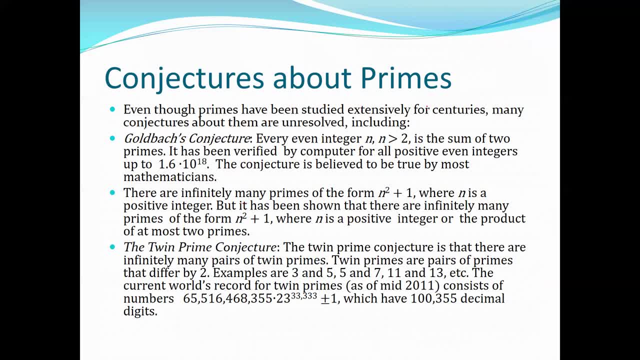 even though prime have been studied extensively for centuries, many conjectures about them are unsolved, including a gold batch conjecture, For example. it says every even integer N and greater than two is the sum of two primes. So it has been verified by the computer for all positive, even integers up to 1.6 into 10, raised to the power 18.. 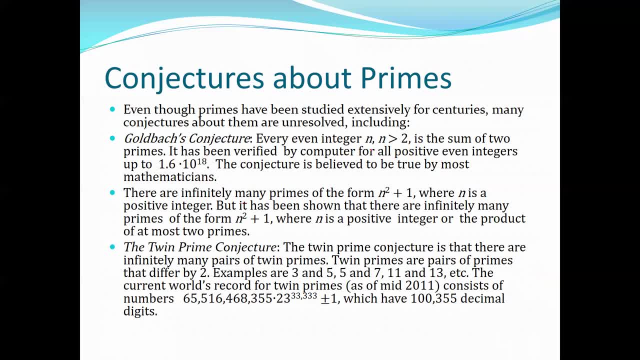 That conjecture is believable to be true by most mathematicians. So it says that every prime greater than two is the sum of two prime numbers, For example. for example, if you take seven, so seven is the sum of two prime numbers. 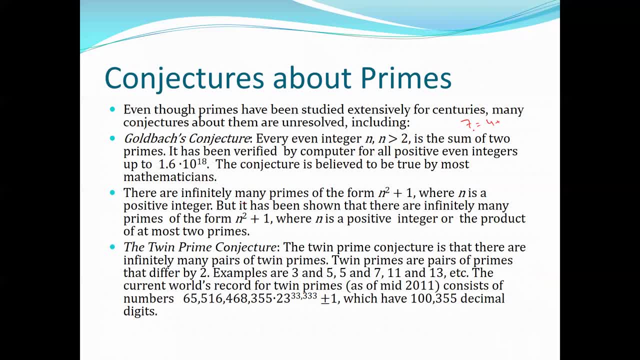 That is uh, uh, uh, uh, okay, Sum of two prime. Okay, Every integer N site, every integer N is a sum of, for example, integer. for example, you are going to take a 13. So this is basically what sum of two prime numbers? 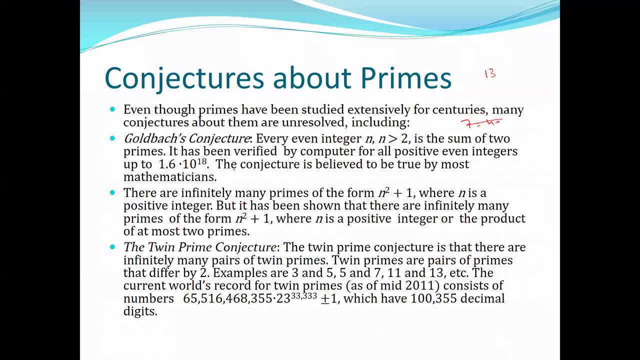 right, Any integer. So uh, and then it it, yeah, we, uh the computer, uh, we have the computational programs. that has proved. and the verified verified this conjecture right. Let's say, for example, 20,. 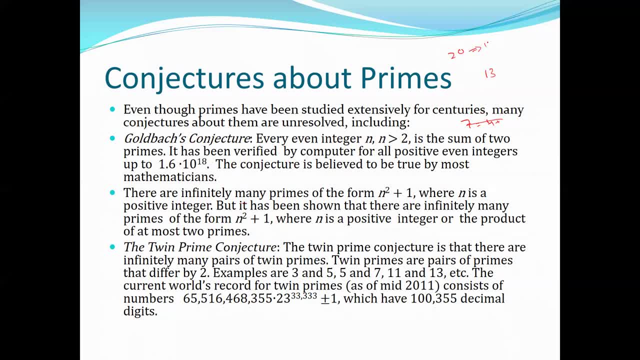 20 is a number that is greater than two. That is some of two prime numbers. That is 13 plus seven, right? So both are, uh, the prime numbers. Every example, any number, as a very example, uh, you can take 40.. 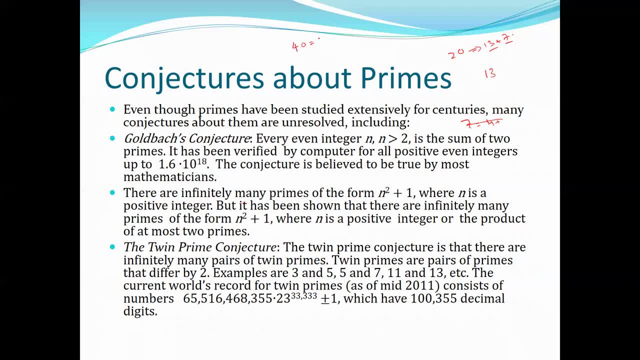 So 40 is some of uh, some of uh. 37 plus three. both are the prime numbers, right? So any, any number that you can take, you can see that, uh, that would. that would turn into the: 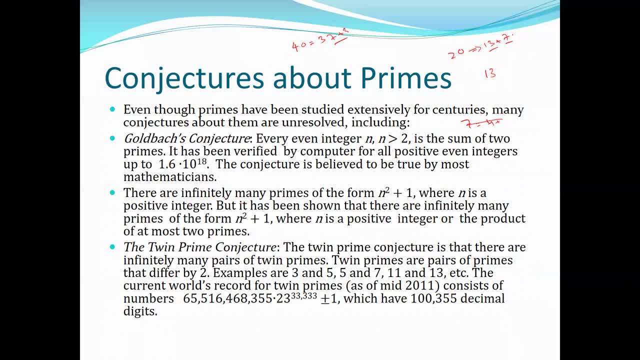 uh prime, uh prime to sum of two primes. There are infinitely many primes of the form and a square plus one where n is a positive integer. but it has been shown that there are infinitely many primes of the form and square plus one where n is positive integer, or the product of at most two integers. 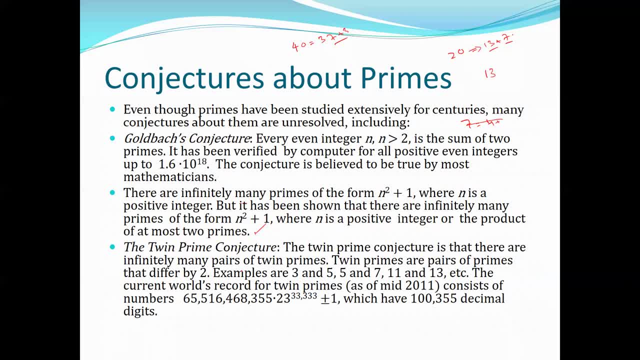 two primes. Yes, right, You can see put substitute the values: the twin prime conjecture. The twin prime conjecture is that there are infinitely many pairs of twin primes. right, Twin primes are peers of primes that differ by two examples at three. 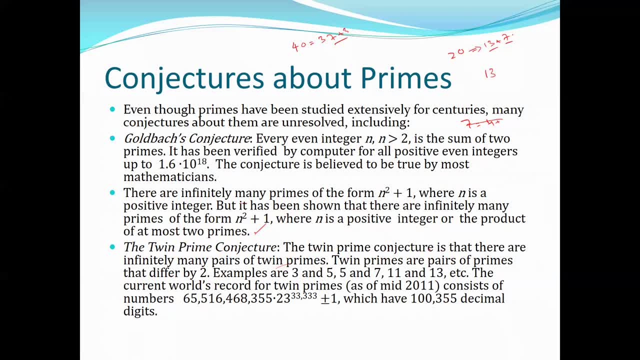 five, five, seven, 11,, 13,, and, and go on. I mean, uh, 17,, 19,, right, And you can see, these are, these are called twin primes. They, they differ not more than two. 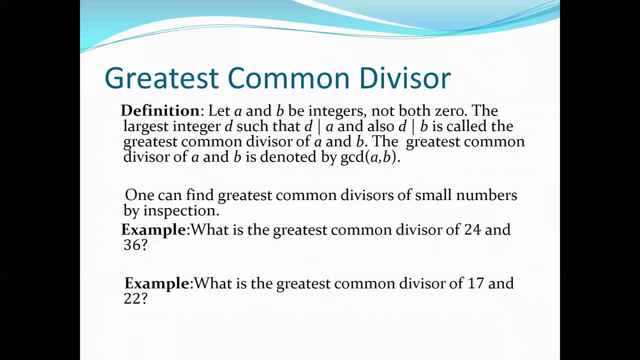 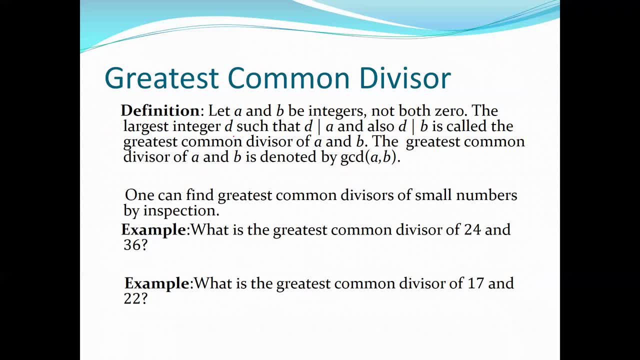 So let A and B be integers. So let A and B be integers, Not both zero. The great, the largest number, D, such that D divides A and D divides B as well, is called the greatest common divisor. Remember, the largest integer right. 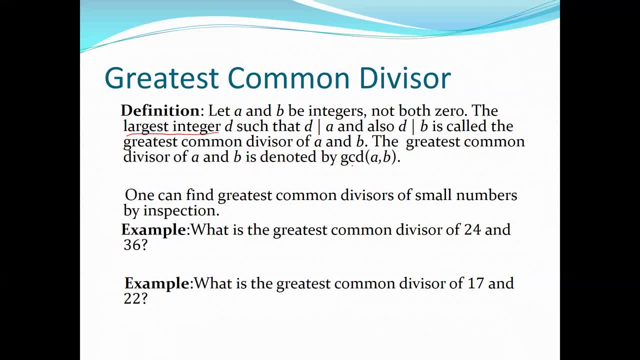 So the greatest common divisor of A and B is denoted by GCD of A comma B, right. So that is how we denote, uh, the greatest common divisor. So one can find greatest common divisor of small numbers by inspection, For example. 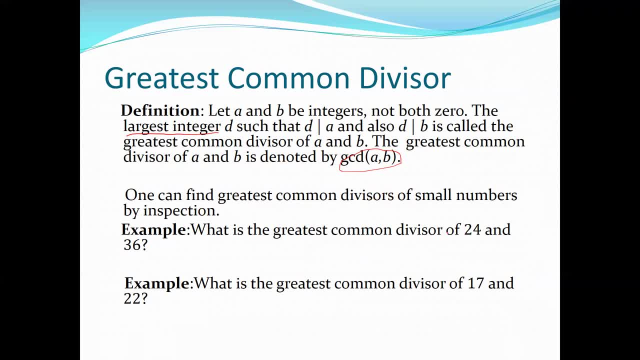 what is the greatest common divisor of 24 and 30?? So we can see that the largest number that divides both is 12.. So 12 is dividing 24, and 12 divided 36 as well. So the greatest common divisor for 24 and 36 is 12.. 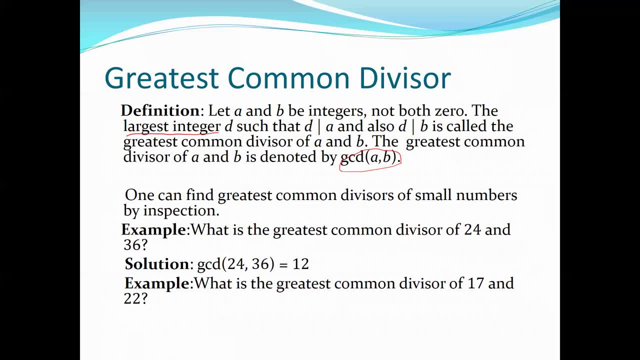 What is the greatest common divisor of 17 and 22?? Do we have the greatest common divisor for 17 and 22?? That is only one. So, um, that is, I mean only one, that is, that divides both 17 and 22.. 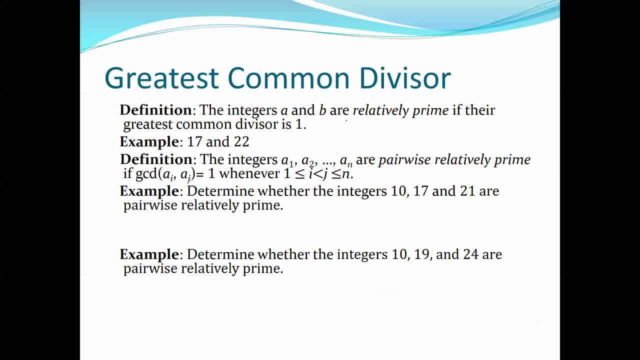 Uh, the uh, okay. Uh, the integers A and B are relatively prime if their greatest common divisor is one. So, for example, if you have 17 and 22,. so they, they, they're common. GCD is one only. 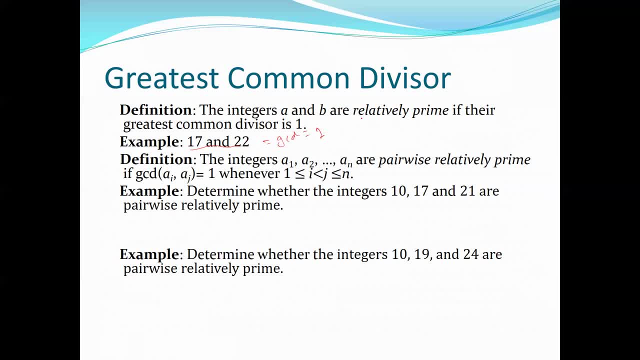 right. So GCD is one. So they are called relatively prime. So one of them is prime, other two both of them are prime right. So the integers A1, A2 up to A and R, pairwise relatively prime, if GCD of A1 comma AJ is one. 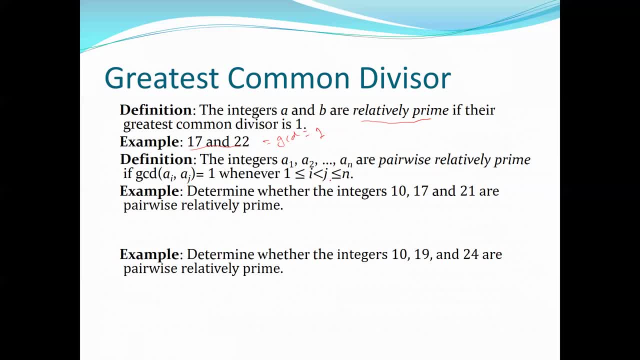 whenever I is greater than or equal to one and J is between I and N, right. So, for example, determine whether the integer 10, 17 and 21 are pairwise relatively prime or not. So what, how we are going to check is because the 10 comma 17 is the GCD of 10 comma 17 is one, and GCD of 10 comma 21 is also one and the GCD of 17 comma 21 is also one. 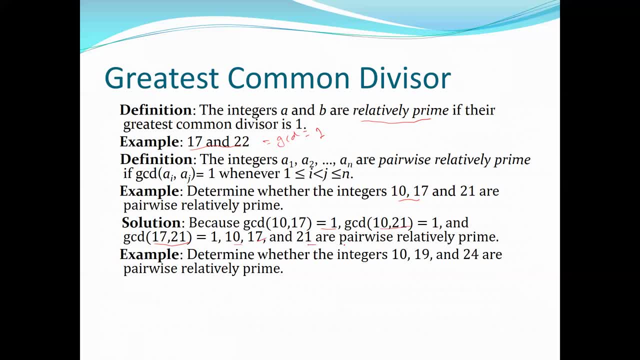 So therefore we say that these 10,, 17 and 21 are pairwise relatively prime. So when we can find the numbers where we find the GCD one for all the peers, we say that this is the pairwise relatively prime numbers. So next example is determine whether the integers 10, 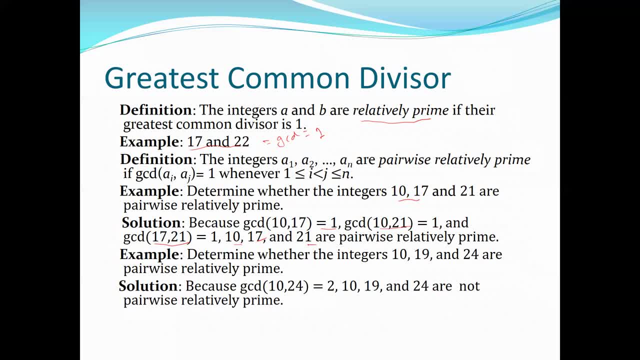 19 and 24 are pairwise relatively prime or not. Since the GCD of 10 and 24 is not one, right, It is not one, So we say that these are not pairwise prime. Simple, clear, Okay. How to find the greatest common divisor. 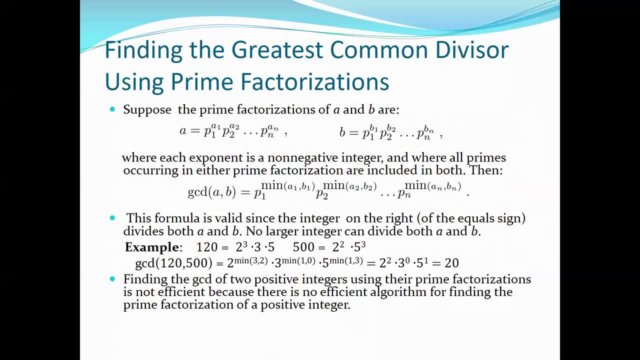 There are different, different algorithms and formulas. One of them is called the prime factorization method. How do we perform the prime factorization? We have understood, or we have learned this in our early classes, I'm sure you. For example, in order to find the GCB of 24, 36, how to do that? 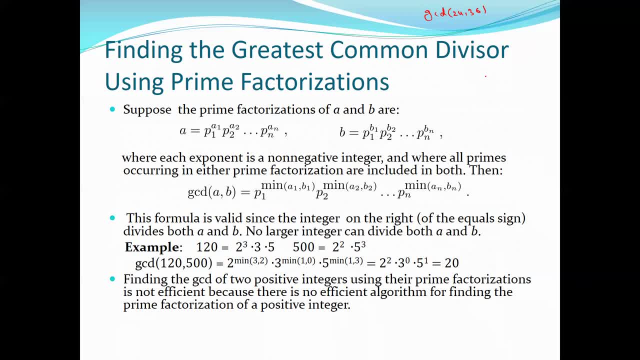 So we have seen that in our classes. I'm just giving you the idea and then we can figure out the algorithm. So what we are going to do is we are going to have prime factors of 24 and prime factors of 36.. So what are the prime factors of 24?? 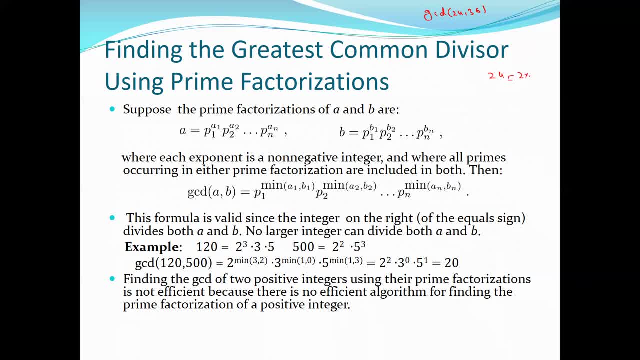 That is nothing but 2 into 2, right. Or you can simply compute the prime factors of 24 like this: 2, 12, 2, 6 and 3 into 3, right. So 2 into 2, into 3 into 3.. 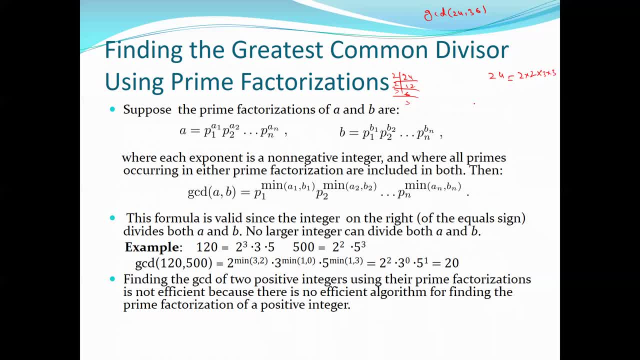 These are the prime factors of 24 and then prime factors of 36.. You can even compute the prime factors of 36 with the same formula: 2, 18,, 2, 9 and 3, 3.. Right. 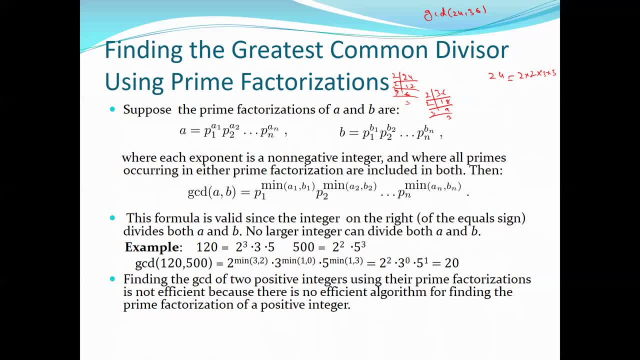 Okay, This is 2.. This is not 3 here. That's what I have: 2 into 3.. And for the 36,, this is 2 into 2, into 3, into 3.. These are the prime factors of both. 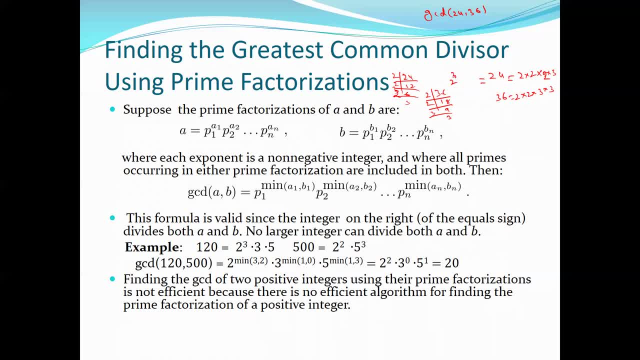 So, if you can rewrite it, this would be 2 power 3 into 3 power 1.. Isn't it Right? And then this could be written. This could be written as 2 power 2 into 3 power 2, right. 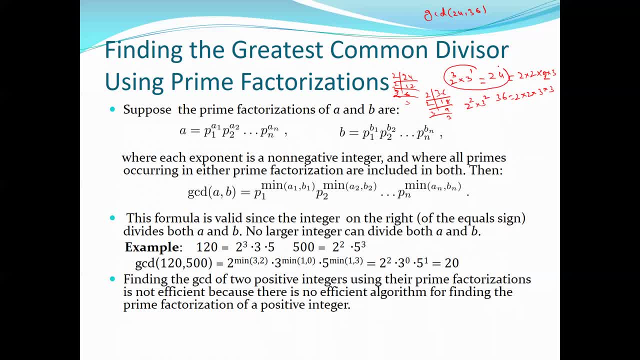 So you have computed the prime factors of 24.. You have computed the prime factors of 36.. Now how can you do that? You can find the minimum of these two, For example. let's see the example here. I mean we have the prime factor of 120 in this way. 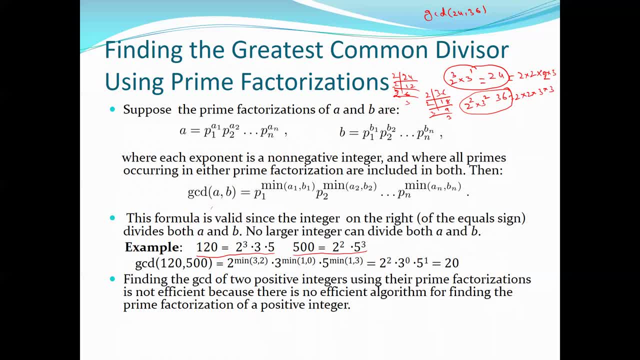 And we have the prime factor of 500 with this. With this I mean these: These are the prime factors of 500. And then we will figure out the minimum out of this. For example, we'll find 2 to the power of 3, minimum of we have two values of 2, 3 and 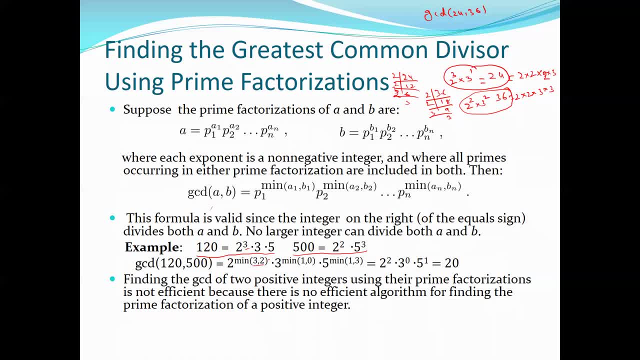 2, right, Which one is the minimum? We'll choose the minimum from them, right? And then we have 3 and we do not have 3.. That means 3 power 0.. So 3 power 1 and 3 power 0, we'll find the minimum out of that. 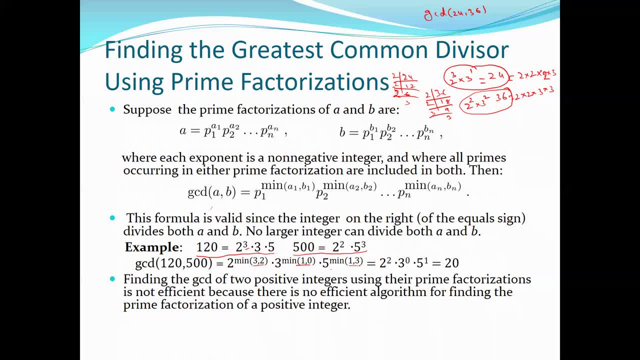 We have 5 on the both side: 5 power 1 and 5 power 3.. We'll find the minimum out of them Right. Similarly, here we have 2 power 2 and 2 power 3.. So we will take the value with the minimum 1.. 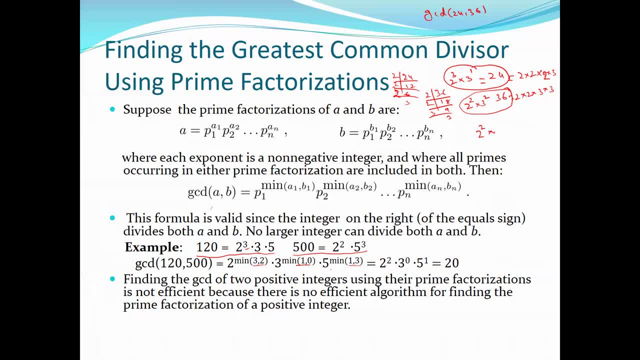 That is 2 power 2.. Right, And then multiply 3. We have 3 value minimum of 3. So 3 power 1 and 3 power 2. The minimum is 3 power 1.. So then it turns out that this is 4 into 3.. 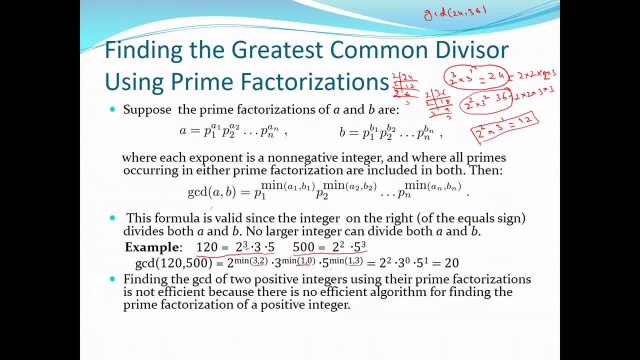 That is 12.. So the prime factor, the greatest common divisor using the prime factor method, factorization method, is 12.. So, similarly, here you have taken the minimum, That would be 2 square plus 3 to the power of 0 and 5 to the power of 1.. 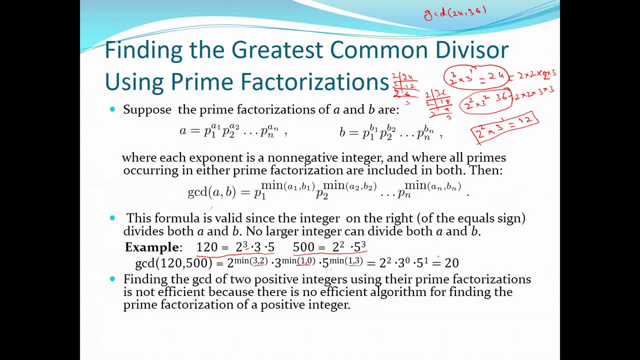 That would be 4, right Into 4, that is 20.. So the greatest common divisor of 1,, 20 and 500 is 20.. Understand So what happens actually if you have a number A with a prime factor of P1,, P2, P up to Pn. 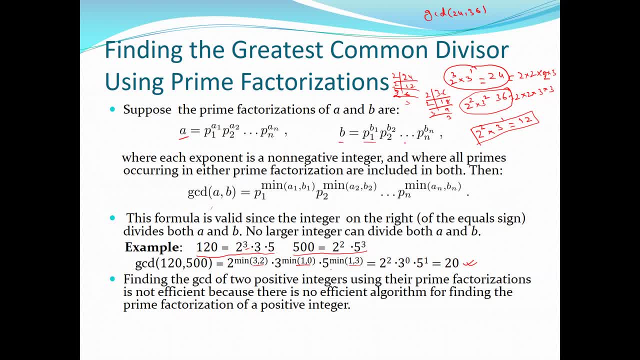 with the power of A and number B, prime factor of P, these prime factors, then what you can do, you can compute the GCD of A, B with the prime factor 1.. In the exponent you will take the minimum value, prime factor 2 with the minimum value. 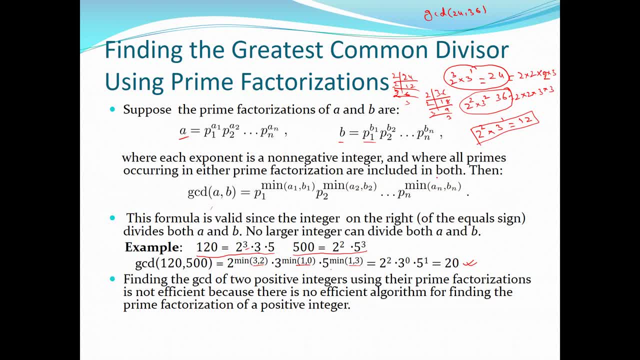 and so on, And I have shown this with an example to you. right, You can rewind the video and see that how we have solved this example and how we have solved this example, And then you will understand Clear, Okay, Finding the GCD of 2 positive integer using their prime factor. 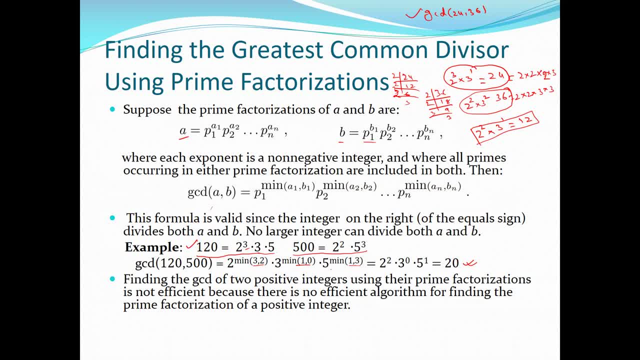 So finding the prime factorization is not efficient because there is no efficient algorithm for finding the prime factorization of the positive integer. So, since we do not have the efficient algorithm to find the prime factorization, so since we cannot compute the prime factorization efficiently, so finding the GCD with the help. 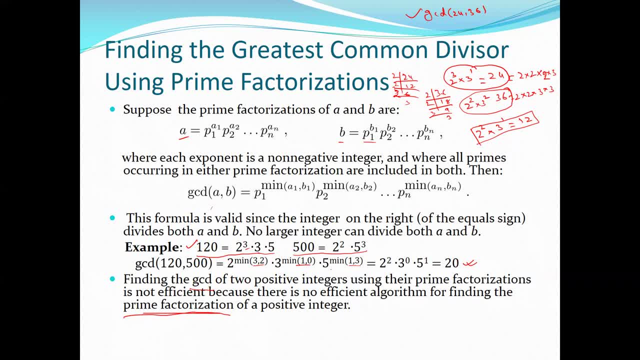 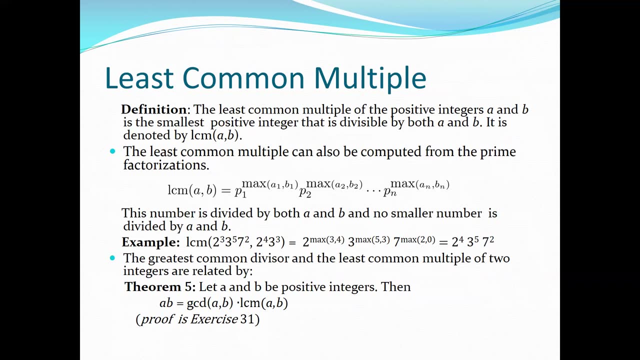 of the prime, factorization is not an efficient way or efficient algorithm. Then let's see what is the least common multiple And then we will see what is the efficient way to compute the GCD or the greatest common divisor. So in the least common multiples we do the same thing, but with the other, I mean we 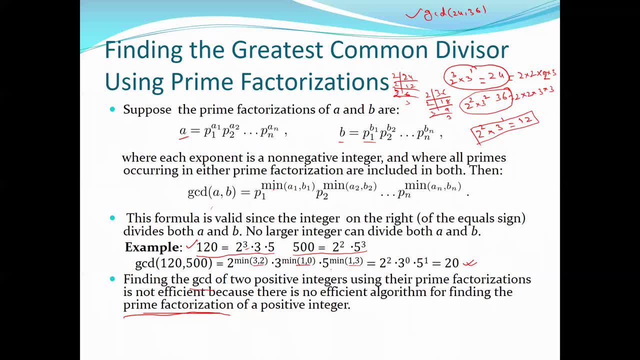 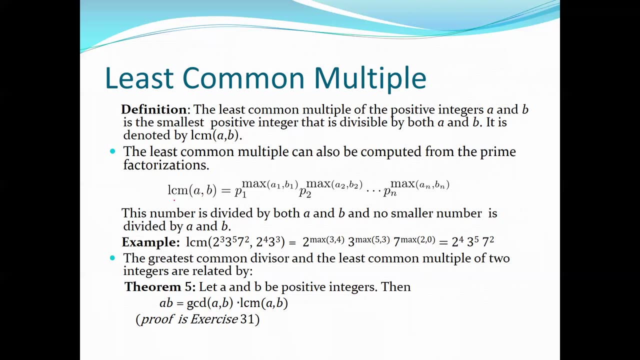 go other way around. Here in the GCD we were choosing the minimum value, right, We choose the minimum of these two, right, And we choose the minimum. But in the LCM, we choose the maximum of these two. See, we have the prime factors and we want to, we are interested to find the LCM. 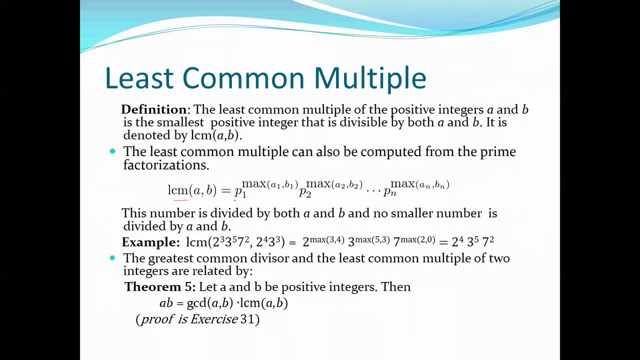 A comma B. So LCM of A comma B is we are going to choose the maximum out of that, So P1, P2, up to Pn, and we compute the maximum out of them. So let's see, Let's see the one example. 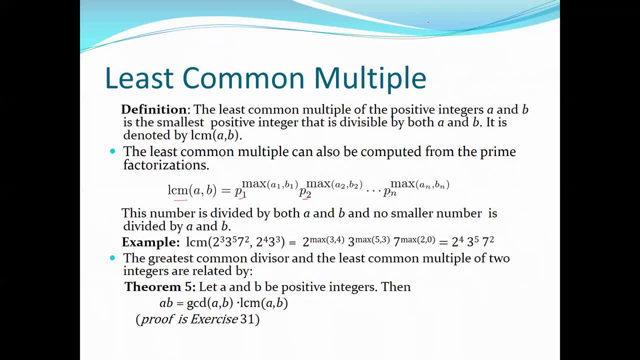 Again we are interested to find, for example, the LC- let me just write it over here- LCM of again 24 comma 36, right The same one. So let's compute the prime factor of 24.. 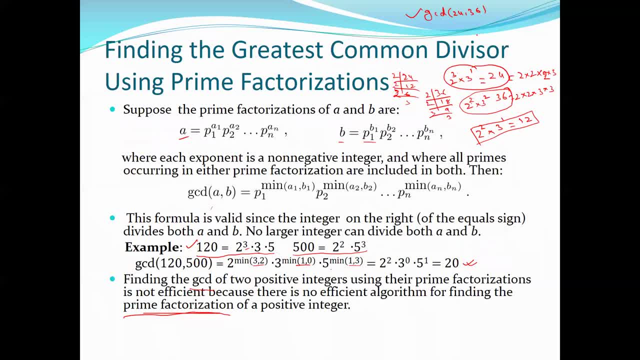 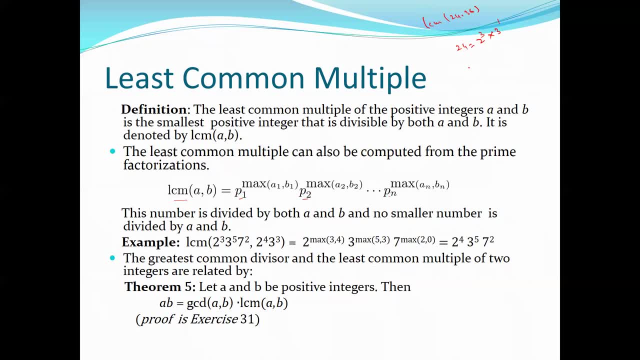 We already know the prime factor, The prime factor of 24 from the previous slide. that is what: 2 power 3 into 3 power 1.. So that is 2 power 3 into 3 power 1.. And the prime factors of 36 is 2 power 2 into 3 power 2.. 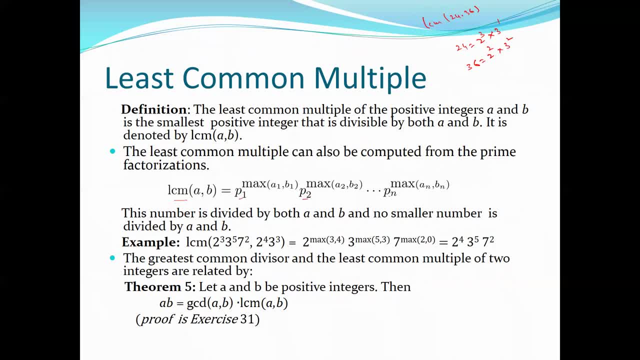 Isn't it See, right, Clear? And the LCM says: choose the prime factor with the maximum. So maximum is 2 power 3.. We will choose 2 power 3 into 3 power 2. Why This is the maximum right. 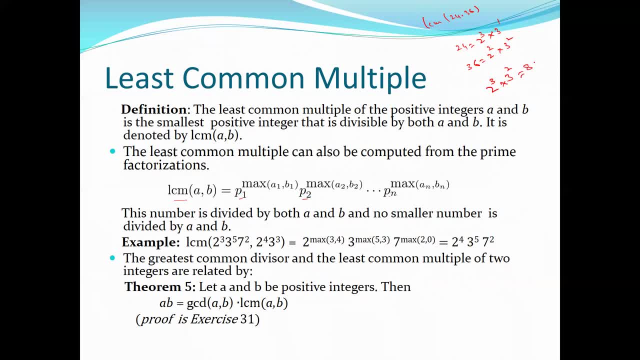 Right And then the this would become 8 into 8, into 9.. That would be 72.. That is the least common multiple right. Clear. So how, that's how we are going to find So LCM of this, these are the prime factors of two numbers. 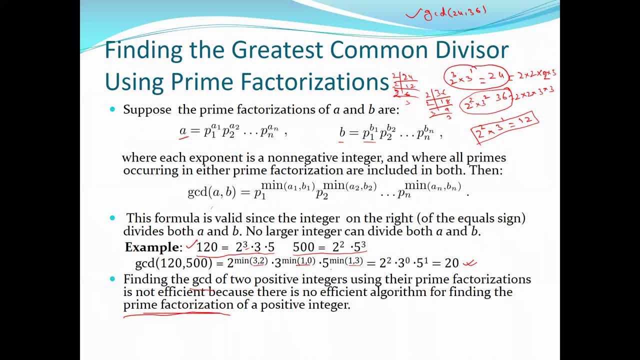 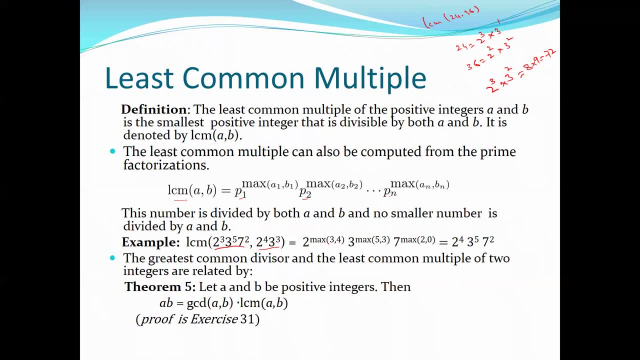 If you remember from here, this is the prime factor of 120 and prime factor of 500, right? No, this is different, This is different. So so you can choose the maximum out of it. So you have to choose maximum, that is 4.. 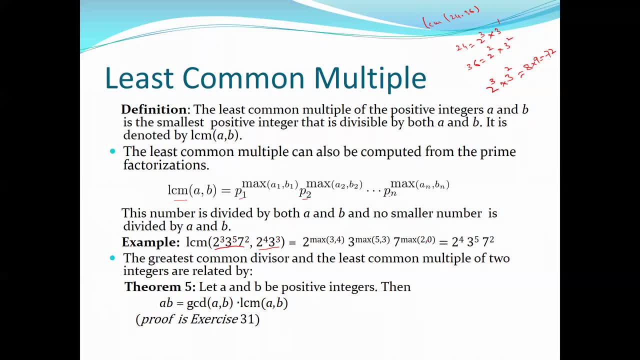 You have to choose maximum, that is, 5 and 7.. You have to choose the maximum right And then this would be the the least common multiple of two integers, right? Okay, So it says that it turns out that the greatest common divisor and the least common multiples 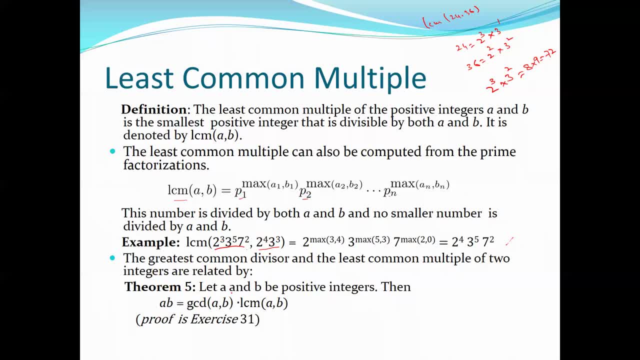 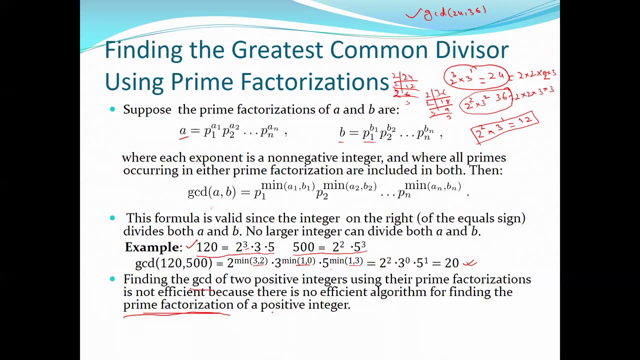 of two integers are related by this theorem. Let L, let A and B be the positive integer, Then A- B would be equal to GCD of A- B into LCM of A- B, Right? So can we? can we relate it here? 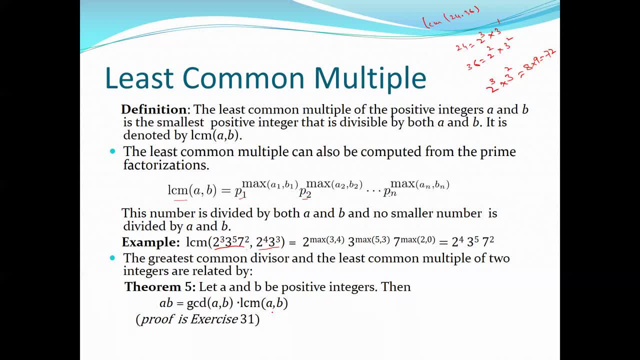 Can we relate it here? Let's see if we can find out. I mean, we can find the number A into B If we want to multiply it. For example, if we want to find the 24 times err Wei 36, that would be equivalent to the GCD of AB that we have found out, that is, 12 into 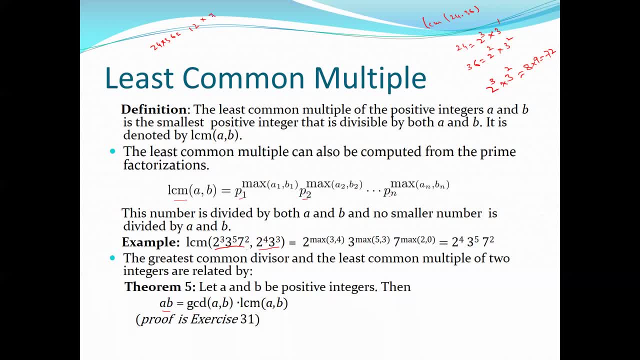 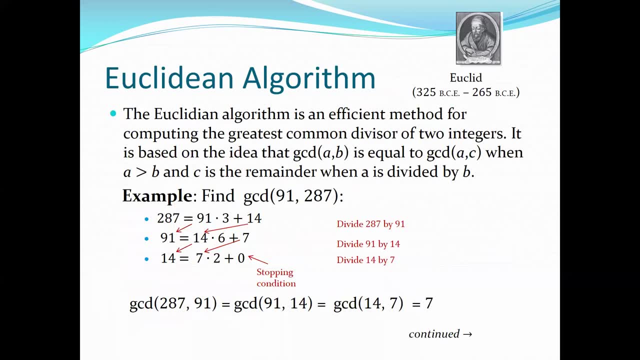 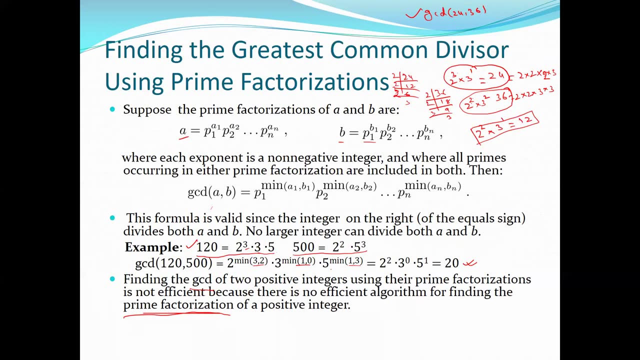 the LCM of AB, that is, we just figured out that is 72. So if you multiply both sides, the answer would be equal. Clear Then, in order to compute, since we have concluded here, the prime factorization method is not an efficient algorithm, efficient way to compute the GCD. 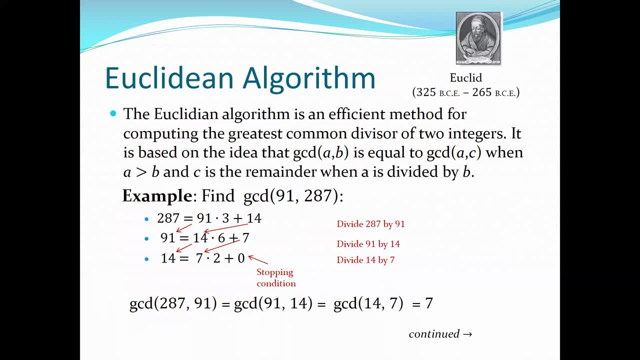 So the efficient method is the Euclidean algorithm. So Euclidean algorithm is used to compute the GCD of two numbers. What does the Euclidean algorithm says? It says: if you are going to find the GCD of two numbers, so for example 91 and 287- understand the concept and then 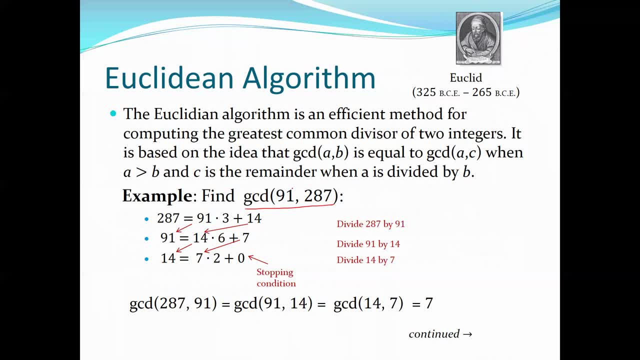 you can figure it out, Then what you are going to do is basically, you are going to find the, the I mean, I mean the. what you will do you will find, you will divide this 287 by this 91. Right, And then you will. 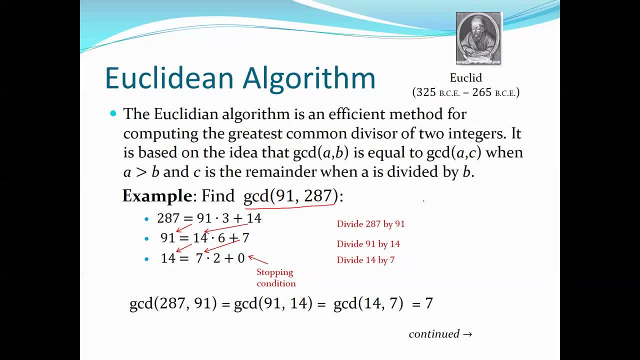 find some quotient and some remainder. We know that if 91 divides 287, right, then we will. it will turn out to the, to the 91, into some quotient plus the remainder, Right? So you will figure out this one. So that's what we are going to do. So, if you are going to find the GCD of two numbers, 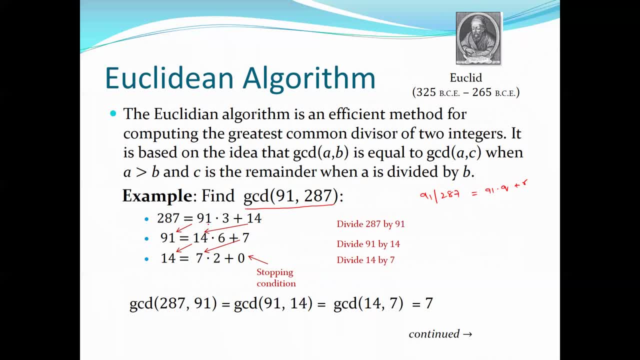 so that's this one, So ninety-one. ninety-one is the dividend, the divisor, Three is the quotient and Loin and 14 is the remainder. And in the next phase, repeat this, Repeat this how: take 91- I mean here instead of 287- and then find out, divide it with the remainder. right, and then you get the quotient reminder again. So what I am going to do is that I am going to say that we are going to divide it by 2. And then we are going to find out a and if the number am you going to unnatural, so that we are going to require the developer? 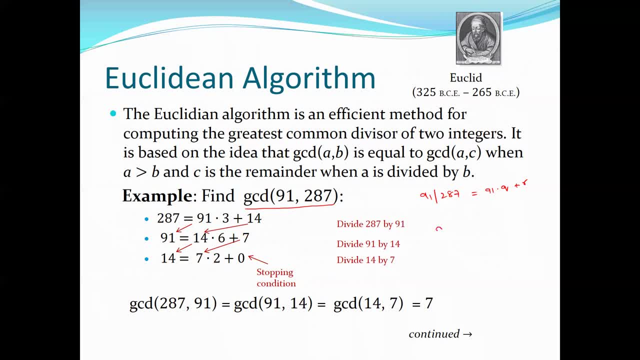 to turn it on the opposites and then I am going to say that 123, keeping course back as I am doing, I am into it here with outside. I mean, is it physicians who want? then clear the general? what happens if you want to find the gcd of gcd of m, comma n, right? so what you will do is: 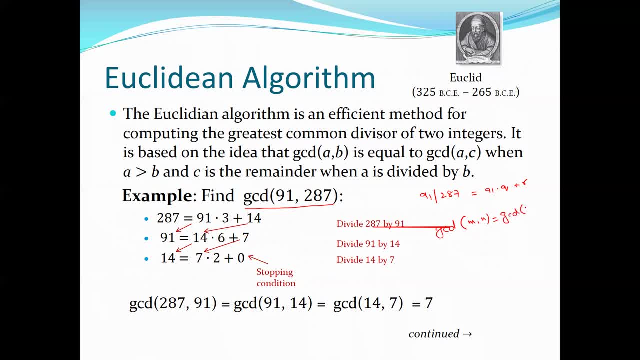 you need to call it recursively: gcd of right, gcd of what, n comma, n comma. what you will do, you will. you will take the n again and then, uh, what you will do, m mod n. right, so that is the divider. uh, then you will get this. if you take the m mod n, you will get 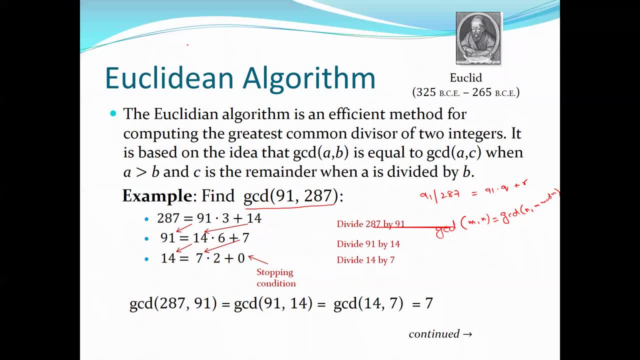 this remainder right, remember uh from the previous class videos. so in order to get the remainder, you need to get the m mod n right. that's what i'm going to say- the remainder. so what i, what actually you are going to do, is first understand this uh first you are going to. this is your uh m value. 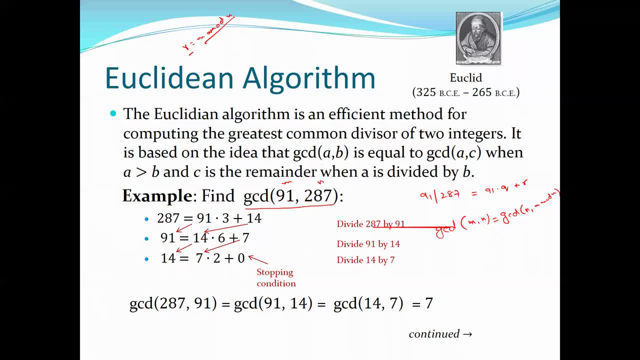 this is your m value, which is your m mod n right. so you are going to get the m mod n right. so this is your n value, right? You are going to divide this n by m right And you get some quotient and the remainder, And in the next step, you divide this number by the remainder. 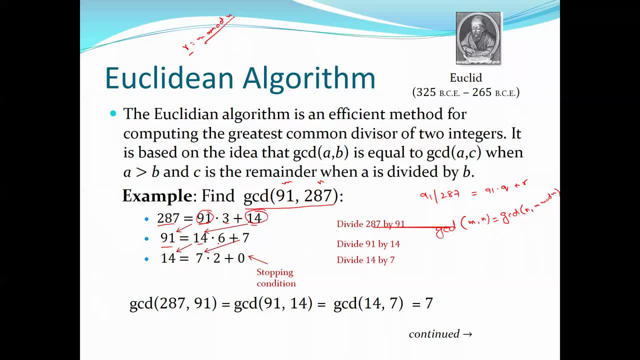 right This number by the remainder and you will get some quotient at the remainder. Repeat this: Divide this 14 by the remainder and you get the quotient at the remainder. So do this until you get the remainder 0.. Once you get the remainder 0,, that means the number is 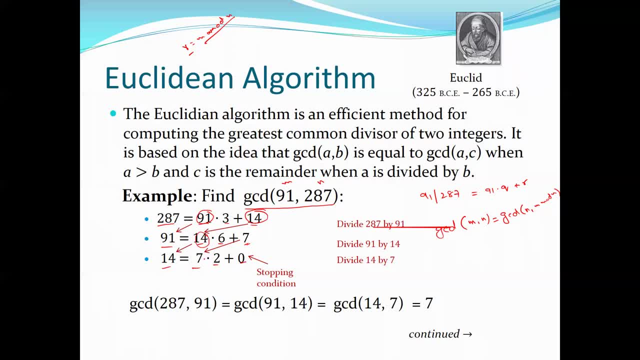 divided equally by this one And whatever is the value you got, the quotient here would be the greatest common divisor, right, See 287 and 91, right, And you recursively call GCD again on 91, with the remainder, That's what I said- the n and the remainder, right, Remainder that you will. 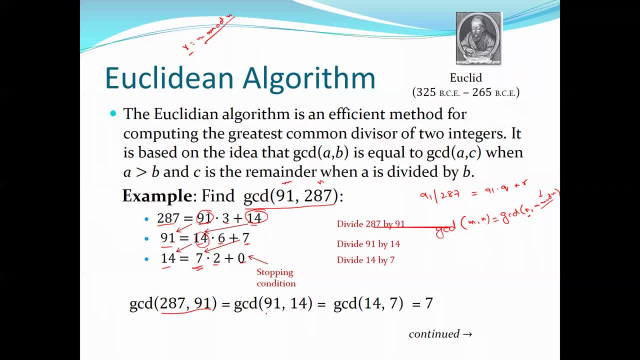 compute with m mod n clear. And then you do, You did this and again you caught. You have to compute the GCD recursively with the 14, that is, this value and the remainder of 91,, remainder 14, that would be 7.. And once you compute, you will go again that you will get 0. 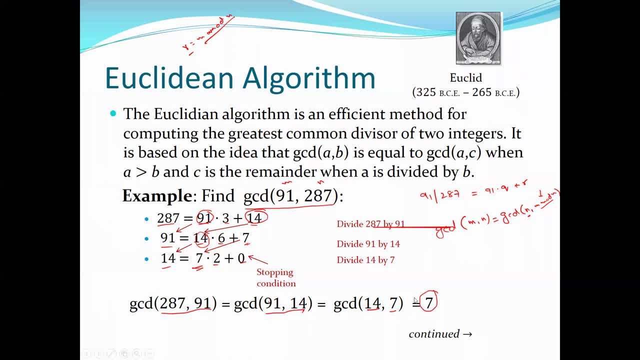 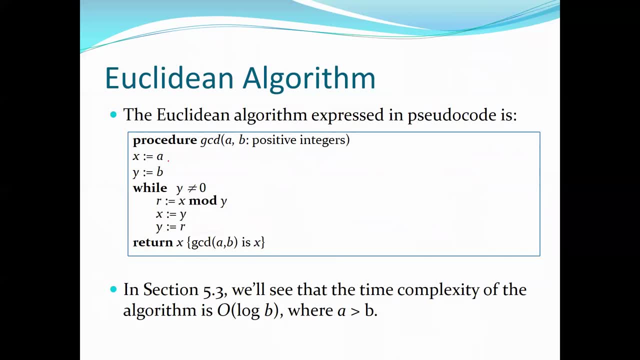 and then that would be the greatest common divisor for this one, That's the Euclidean algorithm. right Here is the pseudocode for this. So the pseudocode is: x is equal to 0.. I mean you are going to take A and B positive integer, You are assigning A to x, B to y, And when you are saying: 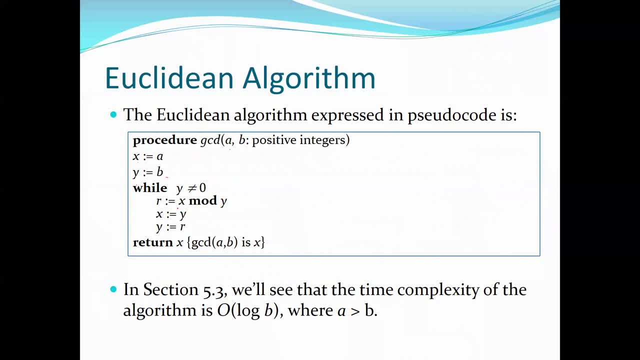 until y is not equal to 0, what you are going to do, you are going to compute the remainder. How you are going to compute the remainder? you know that if you can take mod of x and y, you will get the remainder. And 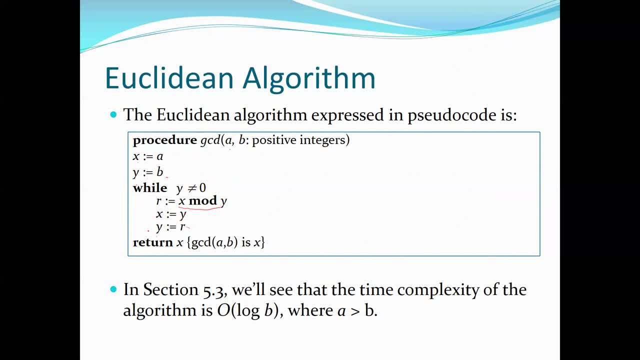 assign the y value to x and remainder to y and repeat it again right At the end, whatever will be the x, the last value in the x, that would be the the greatest common divisor of these two numbers, A and B, based on the Euclidean algorithm. So do. 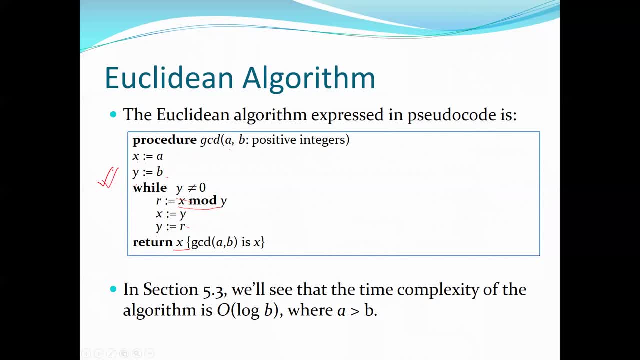 program this in any programming language like C or Java. And then it turns out that the complexity of this algorithm is order of log B, right Where A is greater than B. So what is this? You can prove it. You are already have. we have discussed that- how to compute the complexity, So you can do. 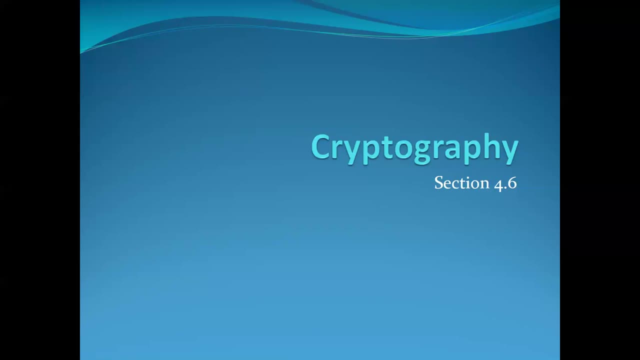 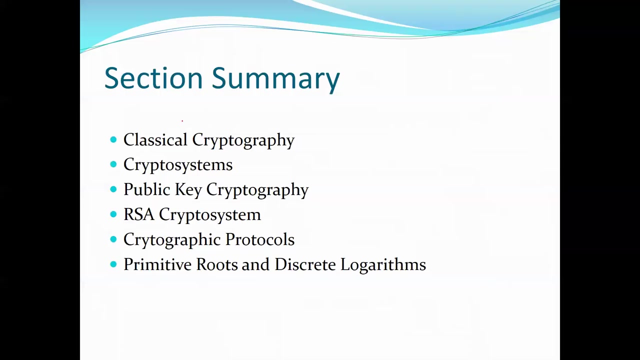 it right. Okay, Now the cryptography. So I am not going to detail the cryptography in very detail, but I mean, there are a lot ofa lot of things that we can discuss in cryptography, like the mystical kurteste cryptography cryptosystems publish. 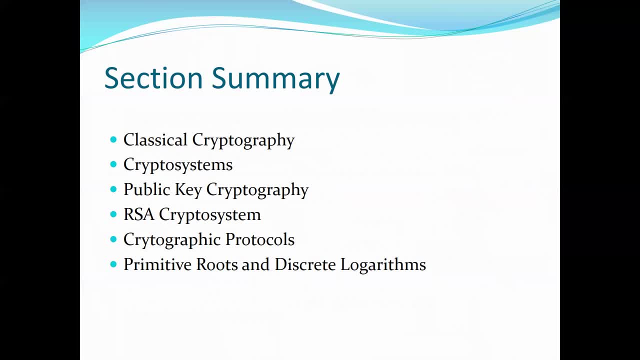 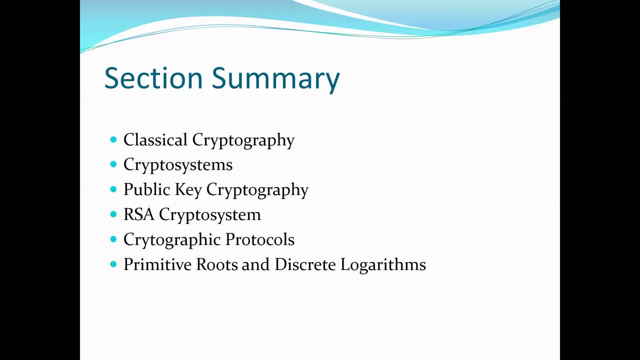 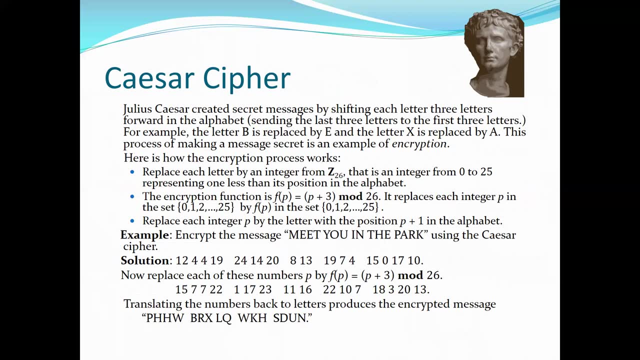 Bye, bye. just give you the idea of the cryptography, that, how the encryption and decryption works and how these are. this number theory, uh, helps in the crypto system. the simplest one is the um the caesar cipher. so this was given by the jealous caesar. he created the secret message by shifting. 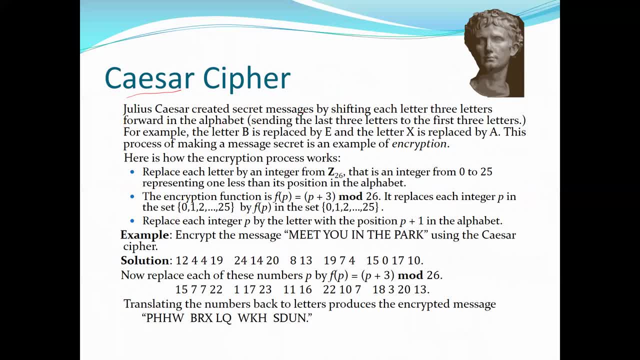 each letter, three letters forward in the alphabet right. so, for example, sending the last three letters to the first three letters. for example, the letter b is replaced with e- i mean b is replaced with e- three letters i had- and the letter x is replaced with a right. so this process of making 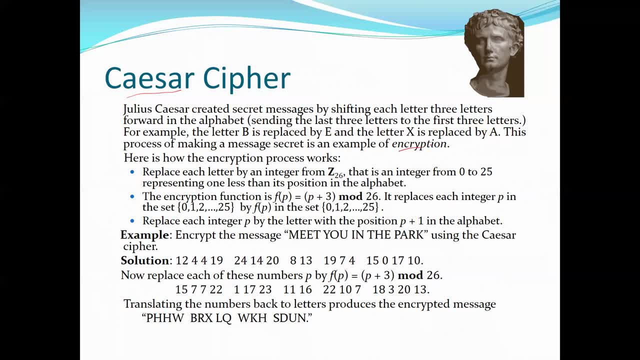 a message secret. um is an example of the encryption right. so here is how the encryption process works for the caesar cipher: replace each letter by an integer. or from z 26. we know that we have the 26 alphabets right, so assign them the value- or from the integer. so, for example, uh a would be equivalent to zero b. 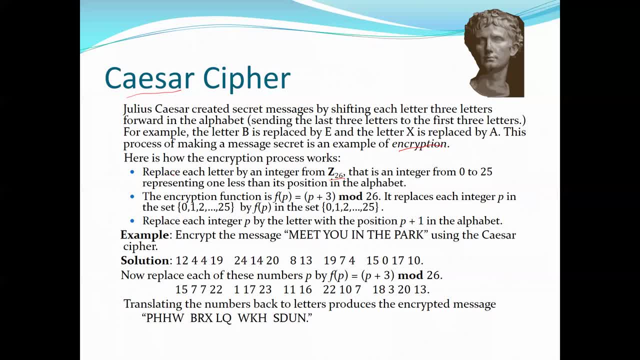 would be equivalent to one, c is two, d is three, and so on. z is 25, right? so then what you need to do is: uh, the encryption function, that there is a encrypt caesars, uh, cipher encryption function that is f, f of p. that what it will do, whatever is the p value, it will add 3 into it and take the mod with 26.. 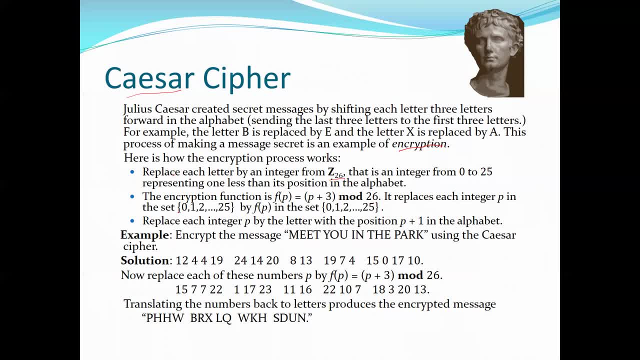 you. so what happens? it replaces each integer p in the set from 0 to 25 that we have just defined by f of p in the set 0 to 25.. so this function will basically give you the value of the next one. so replace, replace each integer p by the letter with the position p plus i in the alphabet. so 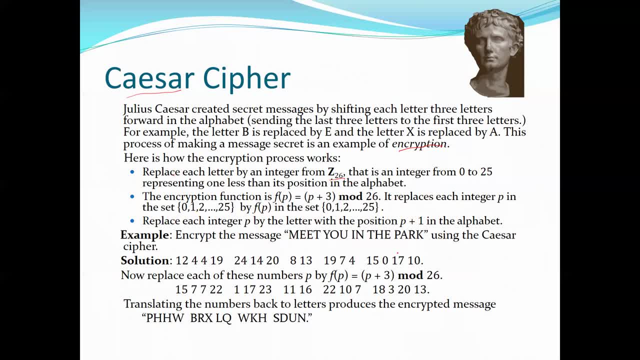 here is an example: encrypt the message: meet you in the part using the caesar cipher. so, if you see m, the corresponding value for m would be the 12, for e is 4, 4 and t is 19, right? so, uh, using this function, what you will do? the p value is 12. 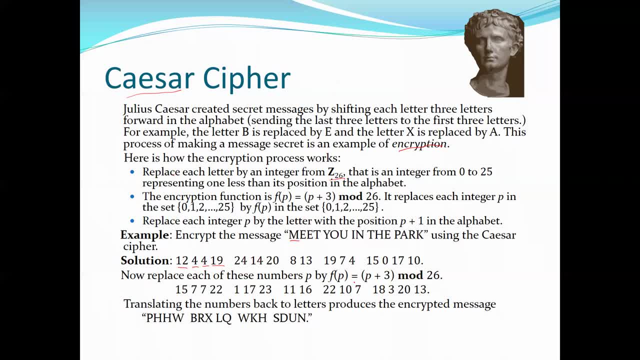 you will get 12 plus 3, 15 mod 26, that would be 15, right, 15 here. 4, 4 plus 3 mod 26 is 4, 4 plus uh, uh sorry. 7, 4 plus 3 is 7. mod 26 is 7. 19 plus 3 is 22. 22 mod, uh, 26 would be 22.. similarly, if you want, 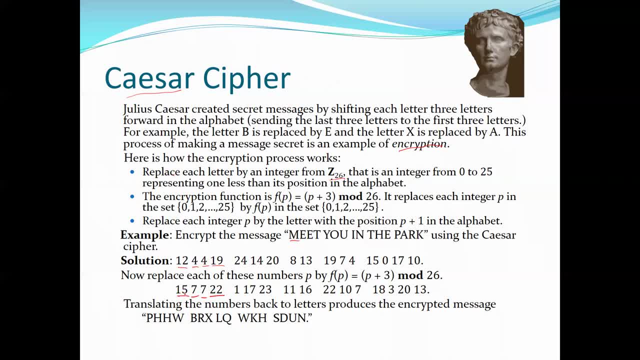 you encrypt the whole message and then it turns out that this would be: p. 15 corresponds to p, 7 corresponds to h, 7 corresponds to h, 22 corresponds to w. here 1 corresponds to b, 17 corresponds to r, 23 corresponds to um. okay, 23 corresponds to uh, l and so on. i mean 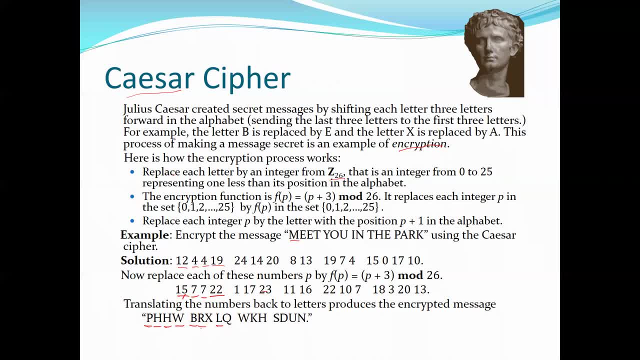 this is how the message is encrypted, in a very simple manner: using this caesar cipher function, right? what is the function? this is the caesar cipher function, right? so, using the number theory, using the divisibility and the modulus arithmetic, we basically in use you, we use this, uh, in the 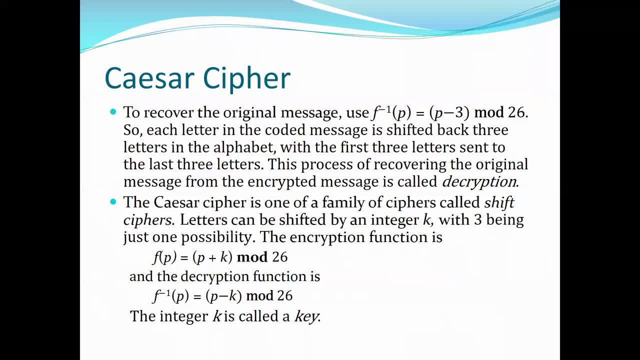 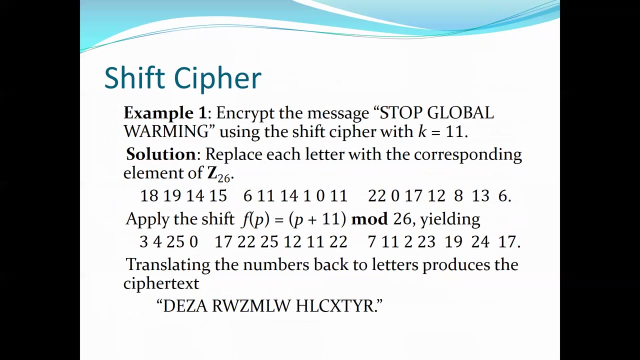 encryption and decryption. so for the decryption or in order to recover the original message, you just take the inverse of that number, that is, p minus 3 mod 26, and that will be decrypted again. so, uh, then i mean we will try it again. For that we can see that there are a lot of functions available for this cryptosystem. 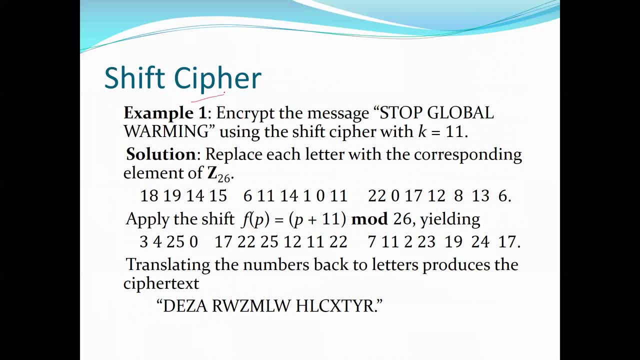 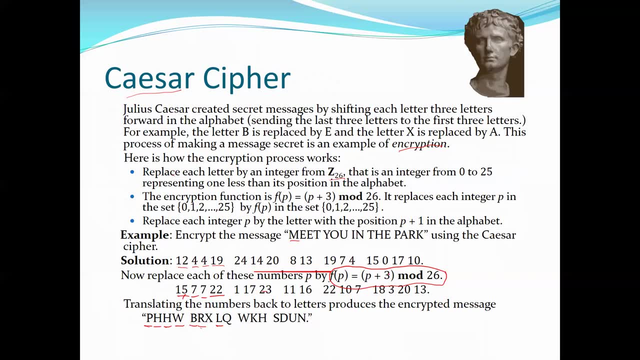 for the encryption and decryption, For example, in the shift cipher you have the flexibility. that why you are going to fix it with the three only right. Here you are going to shift it with three only right. So that was improved with the shift cipher. 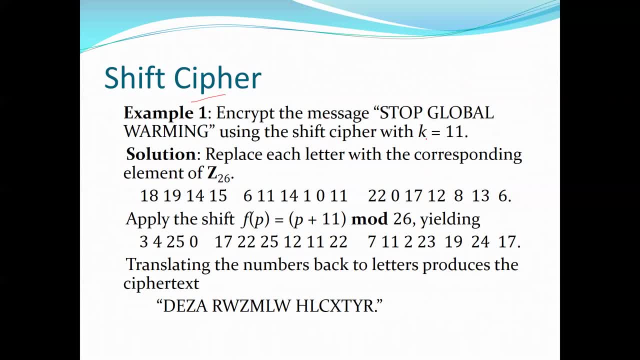 That is why you are going to fix So you can shift it by your own choice. You can give 3,, 5,, 7,, 10,, 20,, 15, whatever you want. So here, if you have, the key value is 11, that you know the person who is encrypting. 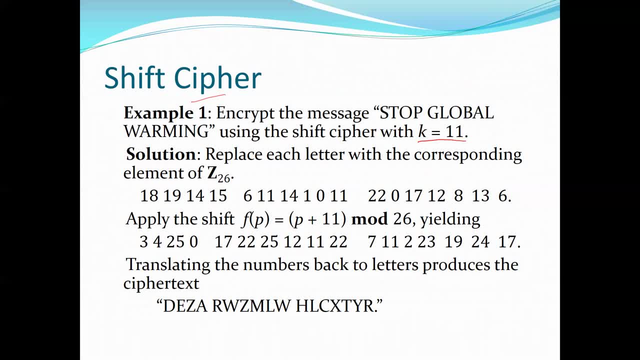 and the person who is decrypting knows that the key value is 11, then you can easily put value 11- and I mean in the function p plus 11 instead of p plus 3, more 26, and then that will be encrypted based on the shift cipher. 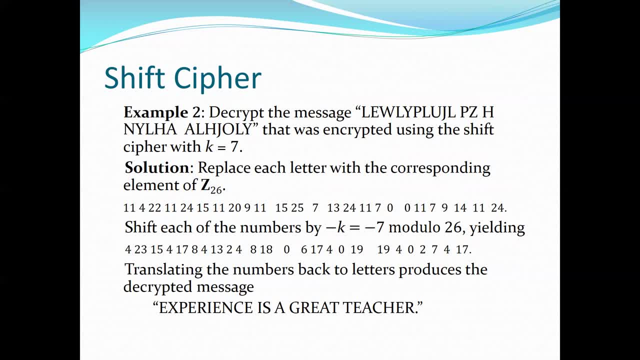 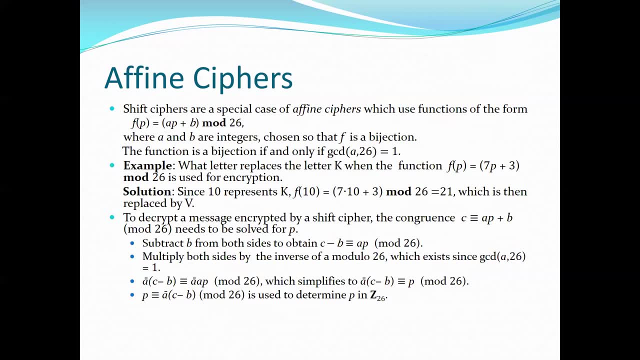 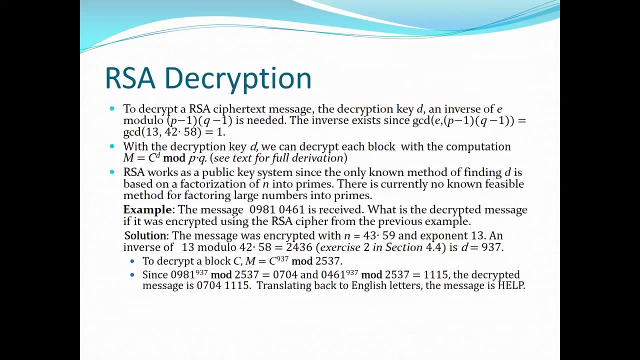 And similar thing will happen for decrypting it. right, In order to decryption, So you need to take the k minus 7, right, And then similar. I mean there are many concepts of find cipher and then the block cipher and the crypto system, RSA, public e-cryptography. 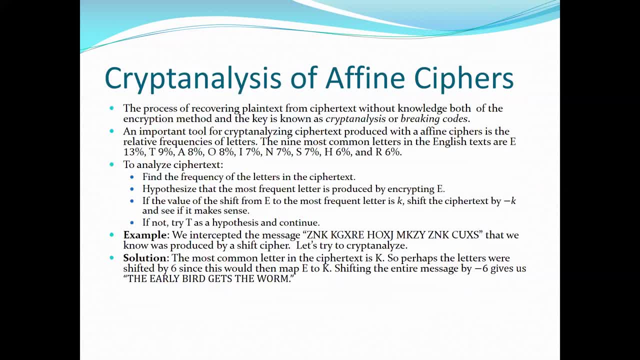 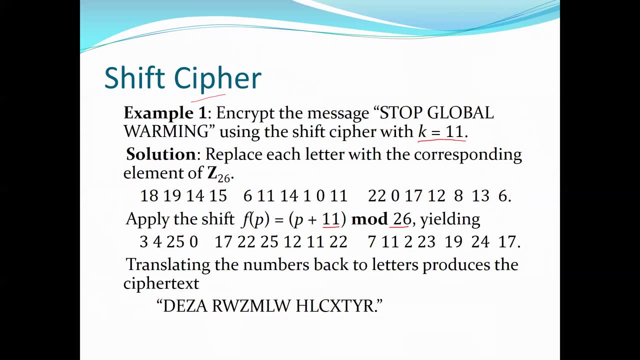 A lot of things are available In this cryptography. that is a separate course, So I'm not going to discuss it. I am going to leave it for your study and for the later semester courses. right? So this was all about the number theory that we have discussed in these three videos. 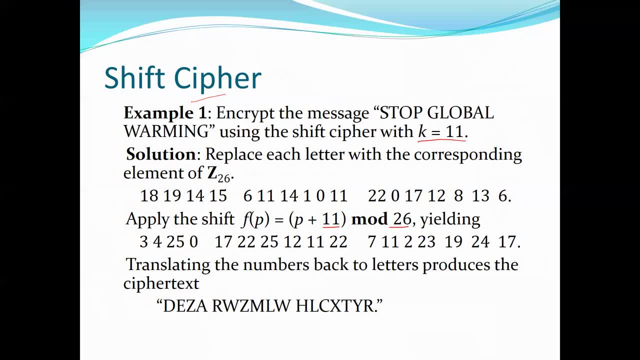 So with this we are ending the chapter number four and we'll come back next week with the new video, with the new topics. All right, Take care and bye-bye. Have a good day.